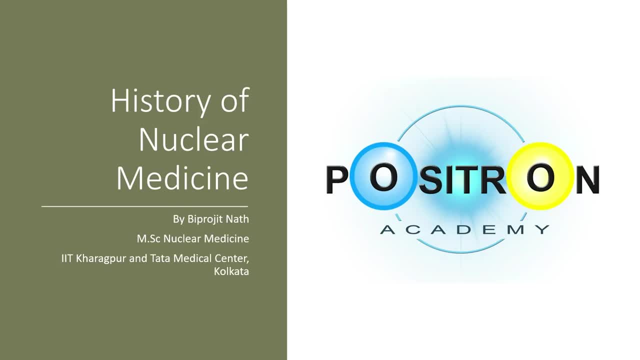 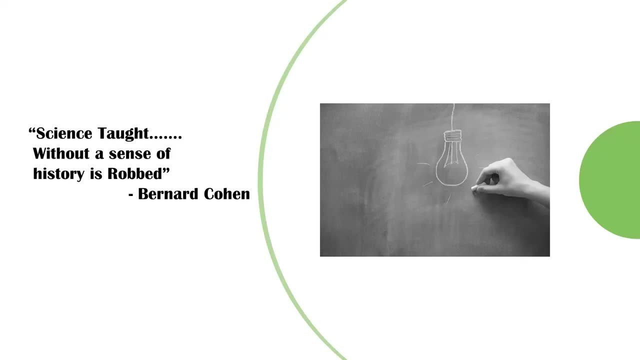 so, hello everyone, welcome to positron academy. and today's topic of discussion is on the history of nuclear medicine. so, as well said by bernard cohen, that science taught without a sense of history is robbed, and that is why today we are trying to understand the history of nuclear medicine. 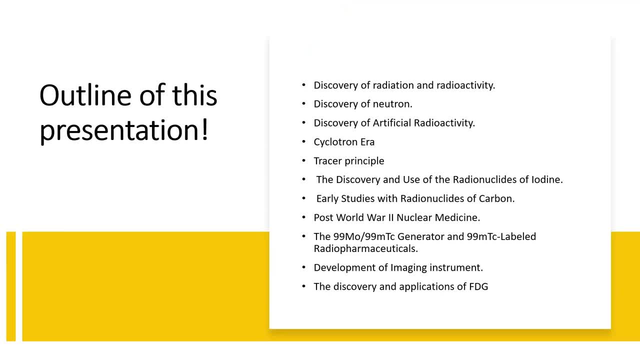 to understand science in a much better way. so that's the outline of this presentation, and we will start with understanding the discovery of radiation and radioactivity, followed by discovery of neutron, followed by discovery of artificial radioactivity, and so on and so forth, in 1895. 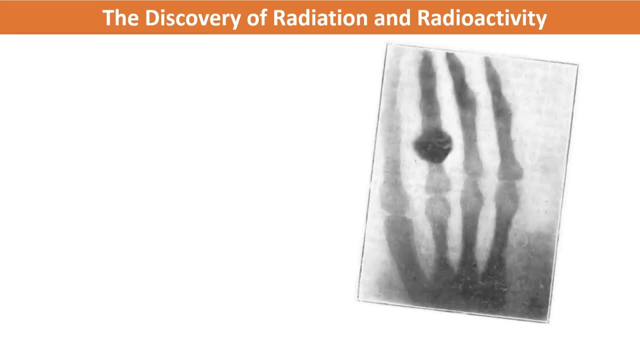 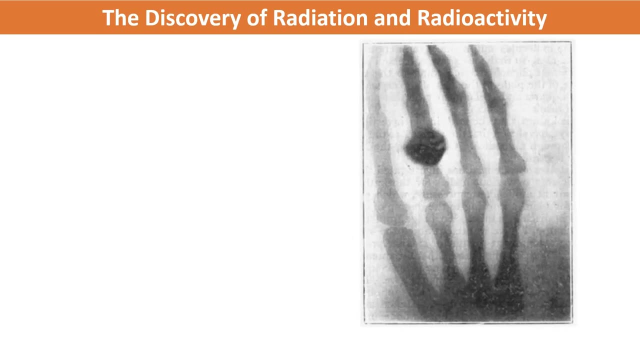 a man took a picture of a hand and this hand picture was so mind-boggling that he owned a nobel prize and he was able to get ronald szerbach and young sure č contrats and has buys a place. it changed the world and his name is william conduit ronjan, and that's the first medical. 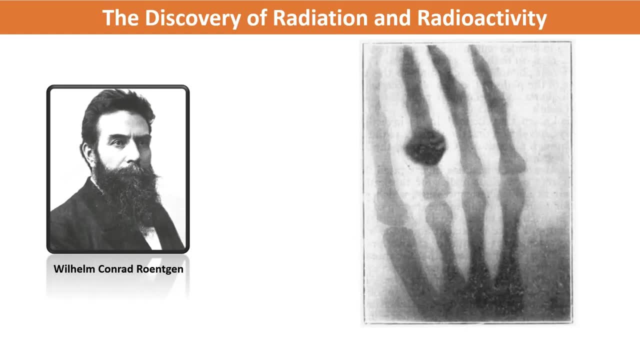 image ever taken may not be very impressive today, but at that time when it was taken was mind-boggling, because it was for the first time we can look inside the human body without having to slice someone open. and indeed medical imaging has changed the face of medicine today. but now the 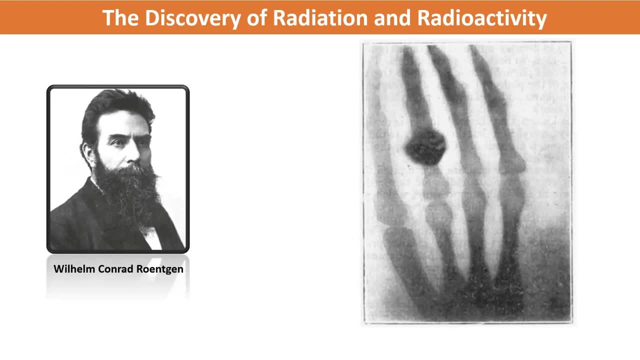 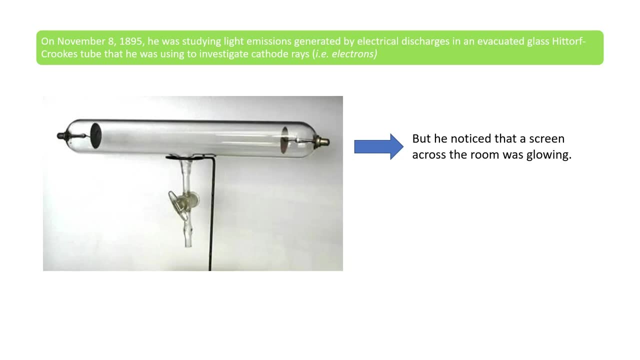 question is how this image was being taken. so on november 8 1895, ron jane was studying the light emission generated by electrical discharge in an evacuated glass hit of crookes tube that he was using to investigate the cathode rays. so he blocked the tube with paper and the room was dark. 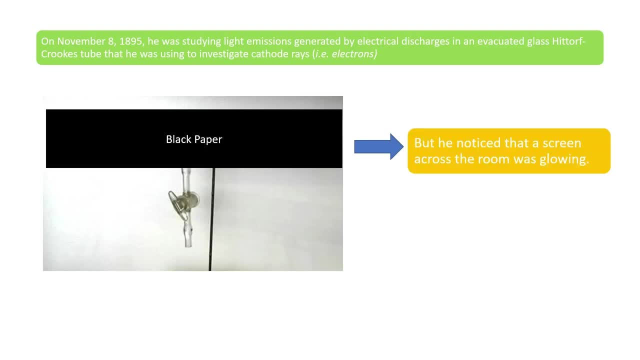 but he noticed that the screen across the room was glowing and when he blocked the beam with his hand, he could see the bones in his hand projected on the screen. and he was very amused. what led to the projection of the bones of his hand on the screen? 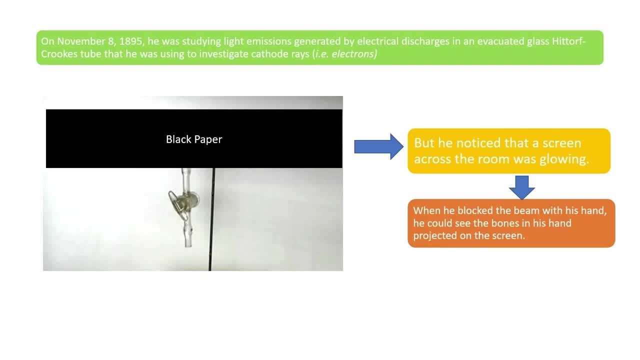 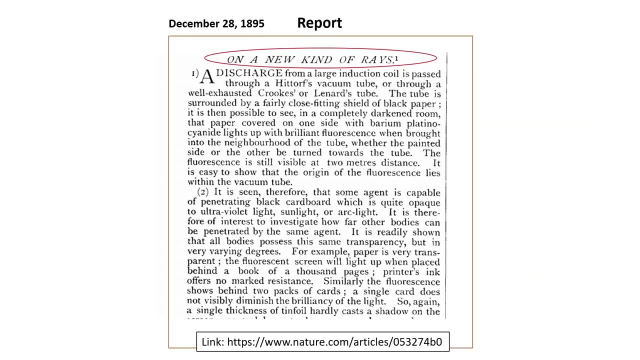 what type of race was being emitted from that particular cathode ray tube, and he spent several weeks studying the new rays emitted from it. so on november also on december 28 1895, ron jane published a report on a local physics committee entitled as on a new kind of race and 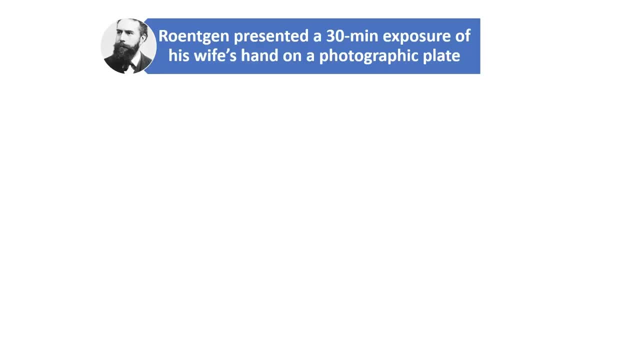 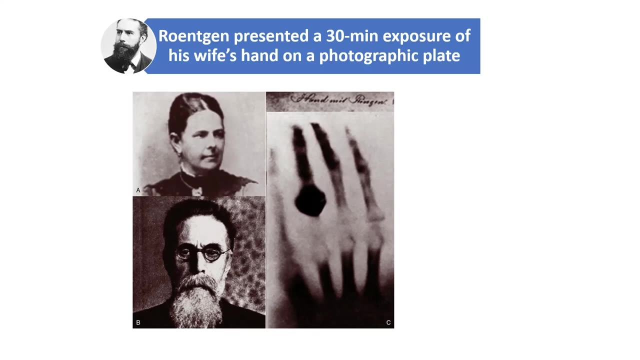 during this committee he exposed, or he presented, a 30 minute exposure of his wife hand on a photographic plate and that's the first medical image ever taken. and that's the hand picture of ron jane's wife, and now we can see how beautiful the image looks like. 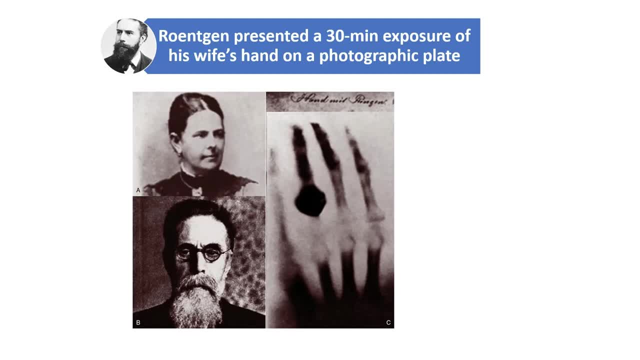 looks so beautiful with the color of tissue and the metal is so clearly visible. may not be the quality is very better, but still whatever we can see in this image is so well appreciated. so by 1896 x-rays were becoming an established tool in medicine, and in 1901, ron jane. 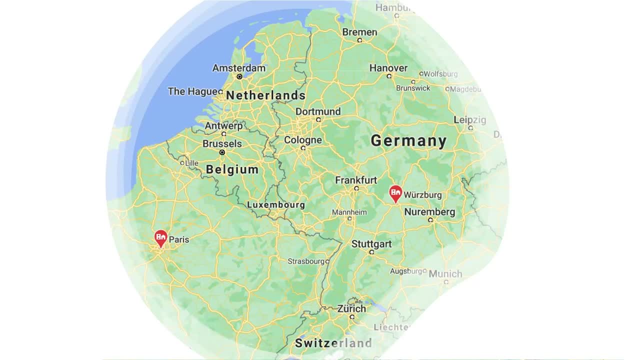 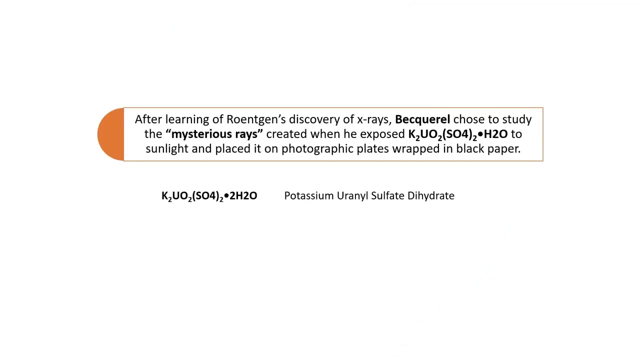 was awarded nobel prize in physics. so that's the georophical map of germany and that's where. that's where ronjen lived at woodsport, and that's in paris where beckerville actually lived. so, after learning of ronjen's discovery of x-ray beckerville, choose to study the mysterious ways. 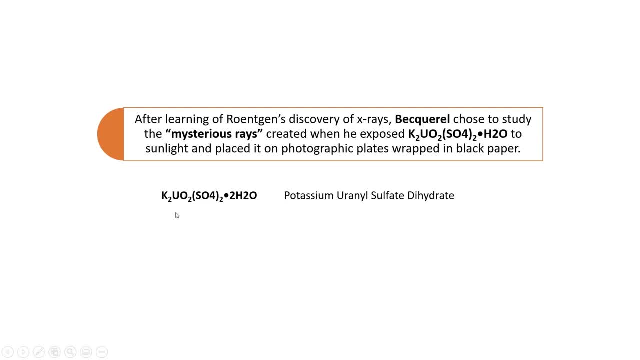 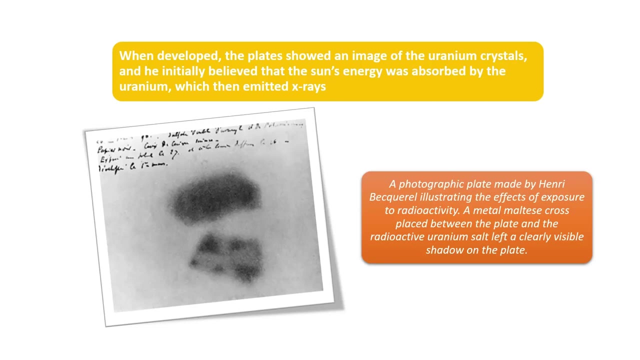 created when he exposed the salt named as potassium uranyl sulfate dihydrate to sunlight and placed it on a photographic plate wrapped in black paper. and that's the impression of which the photographic plate showed of the uranium crystals. so he believed that the sun's energy was. 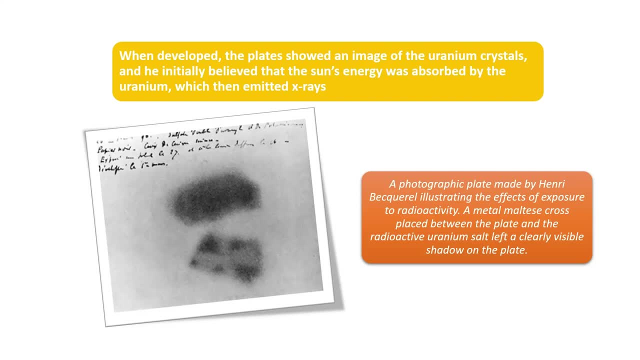 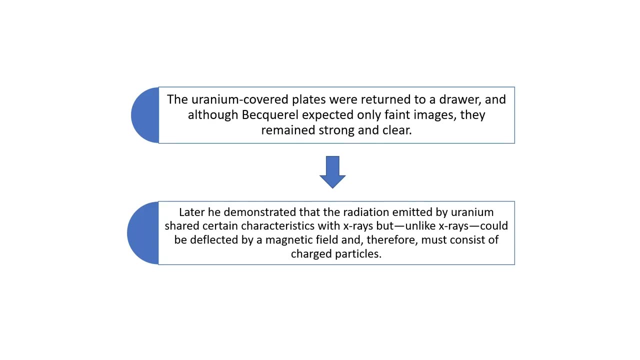 being absorbed by the uranium which resulted in the emission of the x-rays. but later he discarded this belief which he had. so one day this uranium covered plates were returned to a dryer and although beckerville expected only faint image because there was no possibility of sunlight, sunlight in that dryer. 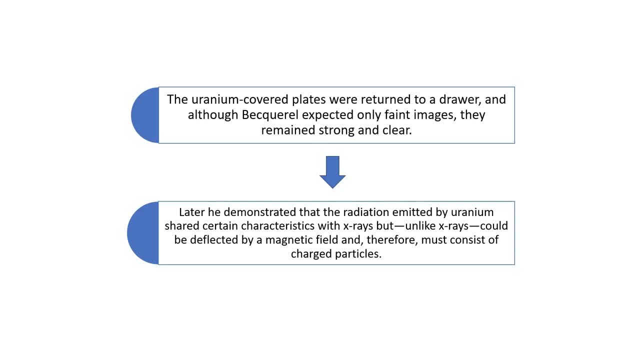 so, but when you open the dryer and you saw, the image remains strong and clear. so that's not related to sunlight, that's something inherent to the, to the uranium itself that lead to the emission of these radiations. later he demonstrated that radiations emitted by uranium it shared. 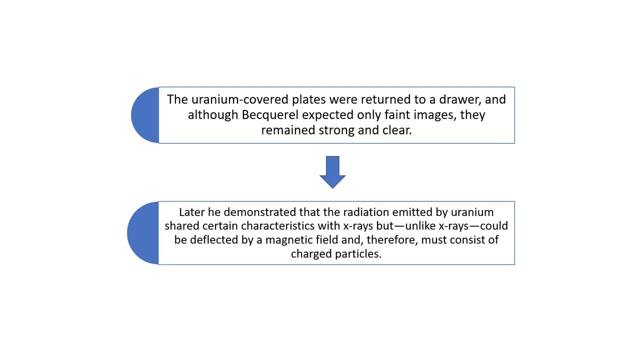 certain characteristics with the x-rays, but unlike x-rays, these radiation could be deflected by magnetic field. so whatever radiation could be deflected by magnetic field. so whatever radiation were being emitted from this uranium, so if these rays, these radiations, were deflected by the magnetic field, indicating that whatever was being emitted by that was charged particle unlike. 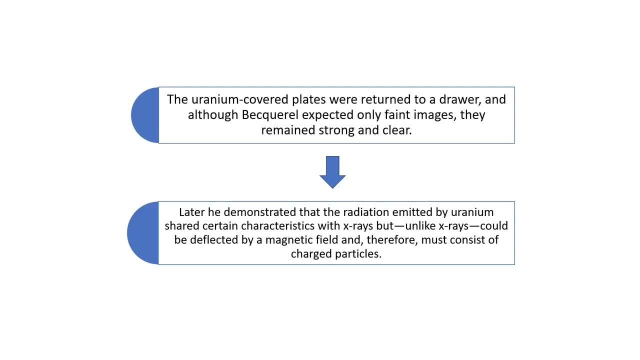 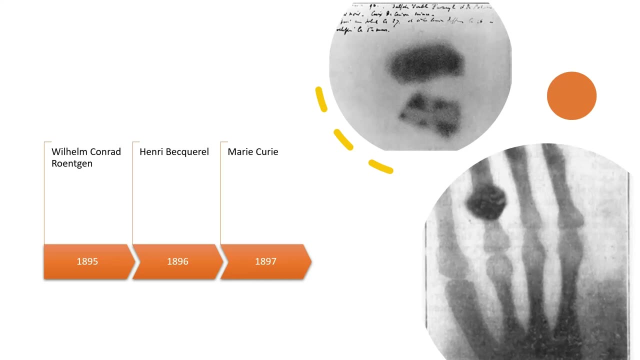 x-rays. these were not deflected by the magnetic field, indicating these were not charged particles. but whatever was released from uranium, these were charged particles as it was deflected by a magnetic field. so now let us see the timeline over here. so in 1895, william conrad rongen discovered 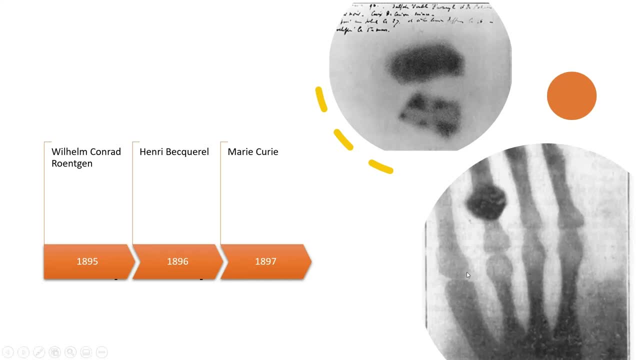 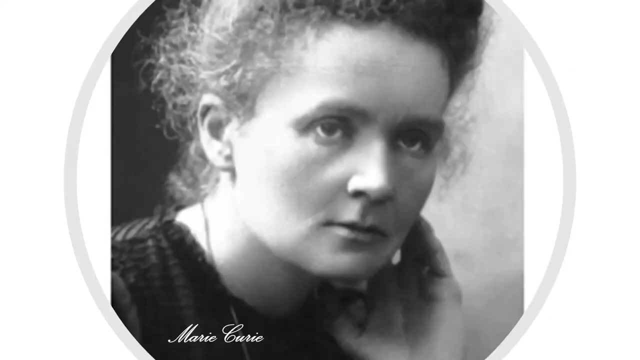 the x-rays and that's the. that's the first medical image ever taken. in 1896, henry beckerville discovered radioactivity. now it's time for medicare. let us have a brief understanding about the contribution, about the roles, about what medicare has done in our tenure. so that's medicare, the name. 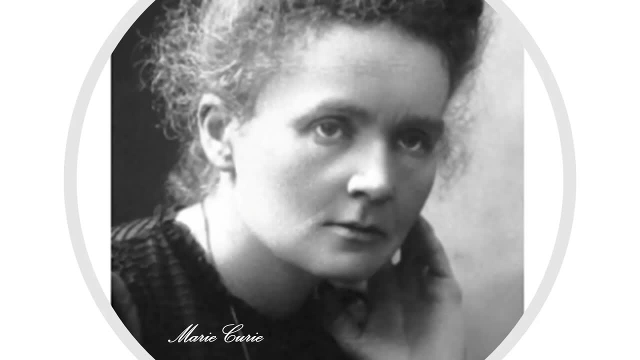 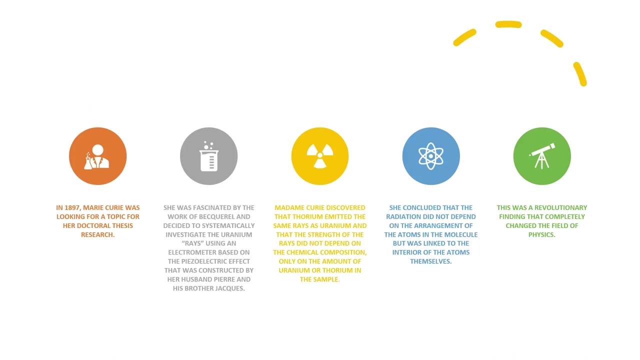 is sufficient and her contribution to the world of um, physics, nuclear physics, uh, oncology is so. it's very mind-blowing. we cannot ignore her name whenever we will talk about radiations, radioactivity, so we have to take her name. so in 1897, medicare was looking for a topic for her doctoral thesis research, and she was fascinated. 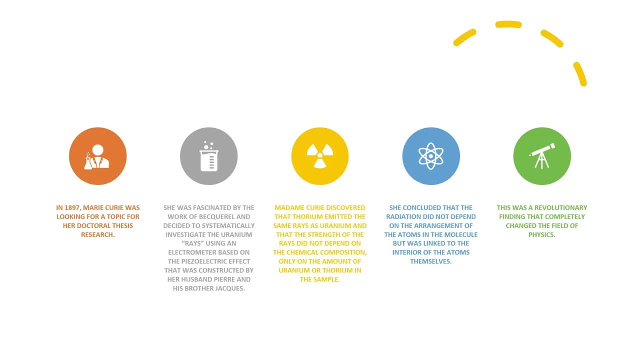 by the word called beckerville and decided to systematically investigate the uh, the uranium rays, using an electrometer based on the piezoelectric effect. and uh. medicare discovered thorium emits the same rays as uranium as as said by beckville, so he she discovered that uranium. 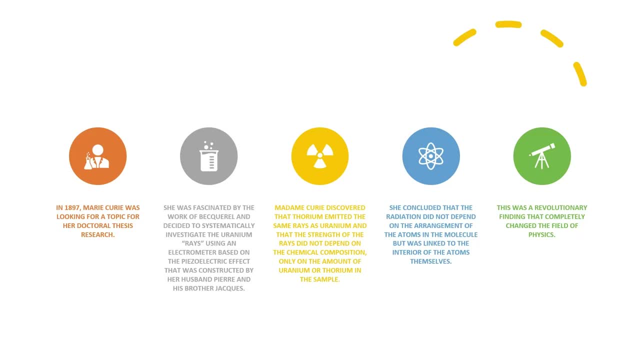 uh. she discovered thorium emitted the same race as uranium, but the strength of the radiation did not depend on the chemical composition. it depend on the amount of uranium, of thorium, in the sample. it means that higher the amount of uranium or higher the amount of thorium, higher will be the radioactivity. 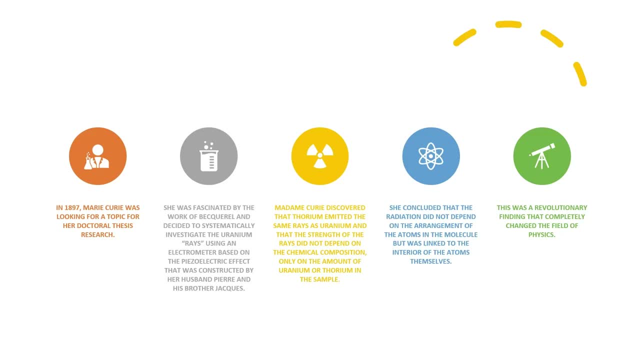 it was linked more on the amount rather on the chemical composition, and she concluded that the radiation did not depend on how the atoms are arranged in the molecule, but rather it was linked interior to the atoms. now we can understand how visionary she was. it, she actually, she actually. 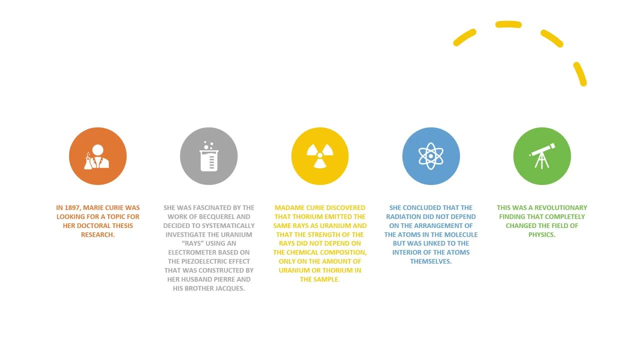 told it much before neutrons were discovered. now we know that neutrons, uh and the n by z ratio, how they regulate the radioactivity or the nuclear stability trend, and she concluded it much way back that the radiation it depends on the interior of the atom themselves but not on the arrangement. 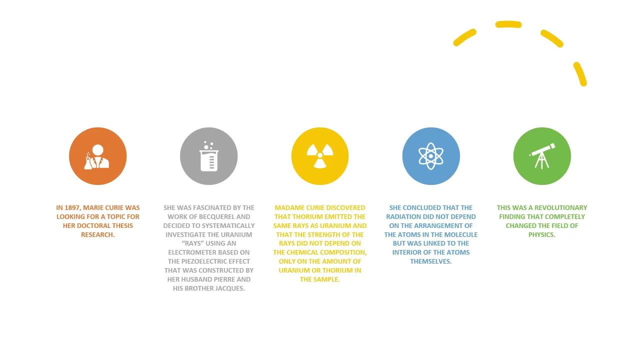 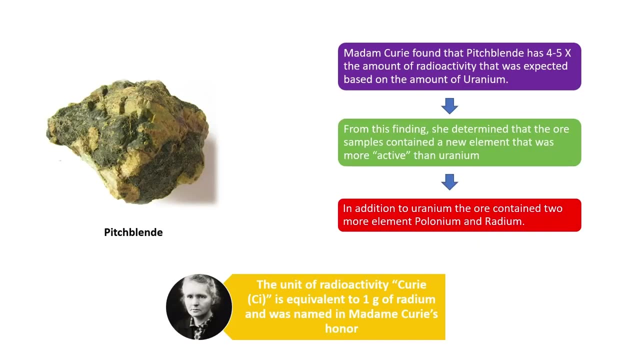 of the atoms in the molecule, and that was a very uh what? that was a very revolutionary finding that actually changed the field of physics, and later on she she decided to work on a very radioactive ore named as speech plant, and she found that the peach plant has four to five times the amount of radioactivity that was expected based on. 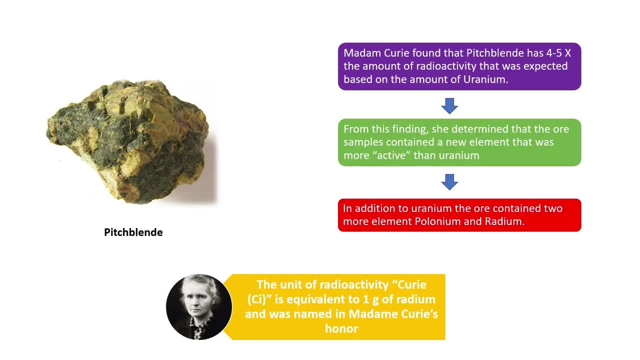 the amount of uranium, so as the, the radioactivity was four to five times higher. so this ore has to must contain some other elements because of which she could get this higher radioactivity. so in addition to um, to the uranium, she uh she discovered two more elements: polonium and radium polonium. 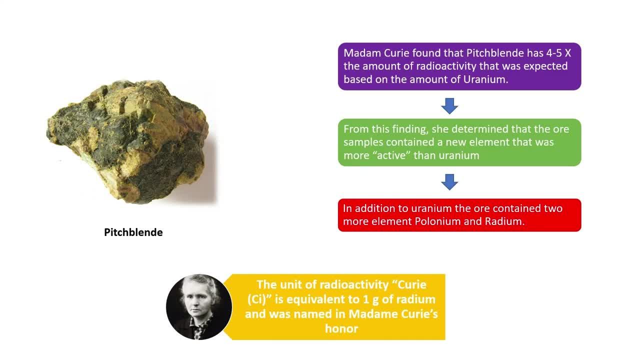 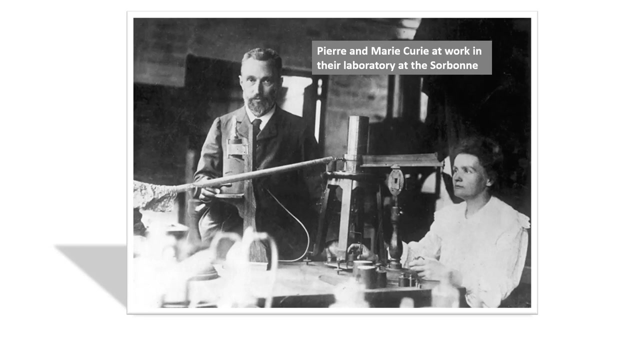 because, uh, because she was from poland, and uh, radium, because that was so much radiative in nature. so the unit of radioactivity- what we call this curie- is equivalent to the activity of one gram of radium, and this was named in madam curie's honor. so that's mary curie in her lab in 1905 and that's mary curie with. 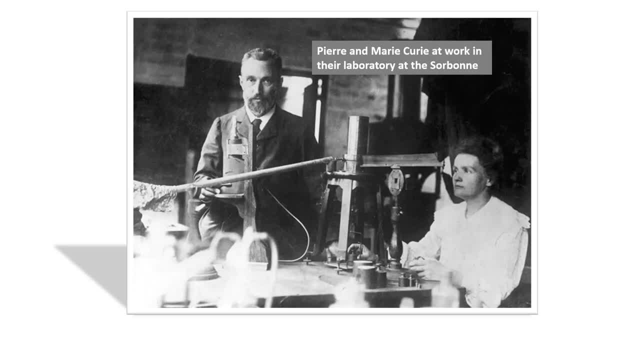 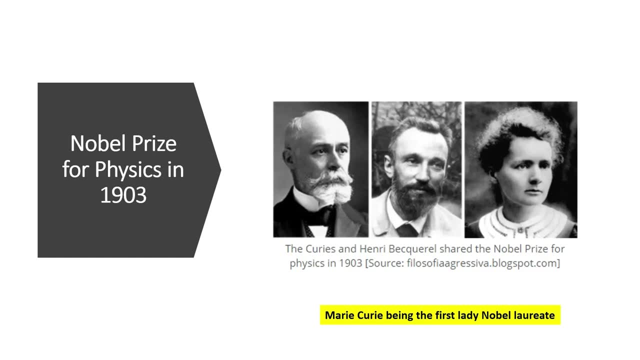 her husband, perry curie, at um at the lab at sorbonne. and and in 1903, um perry curie and hendy beckrell were nominated for nobel prize in physics, but mary curie was being overlooked. but uh, perry could take a stand off of his wife, and then both the curies and 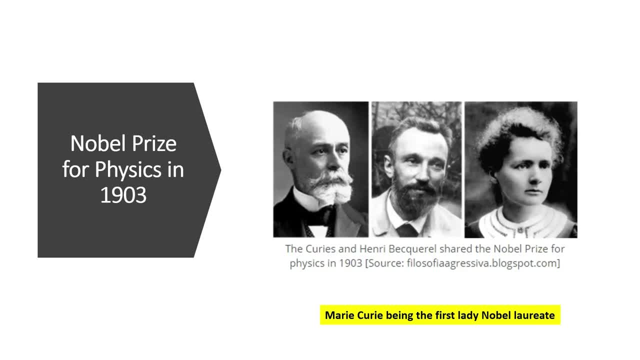 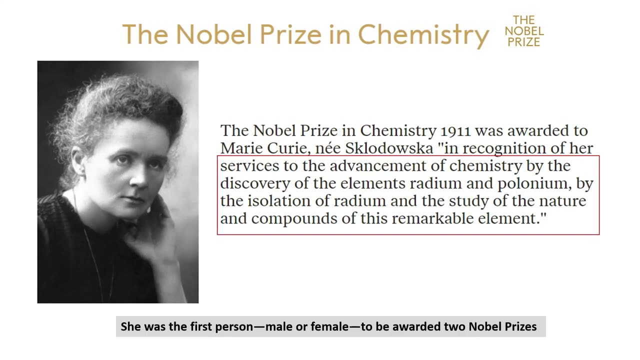 beckrell own the nobel prize in physics and many could be the first lady nobel laureate. so that's the first nobel prize received by mary curie in physics in 1903 and later again in 19: 11 mary curie was again awarded nobel prize in recognition. offered surveys, uh services to the. 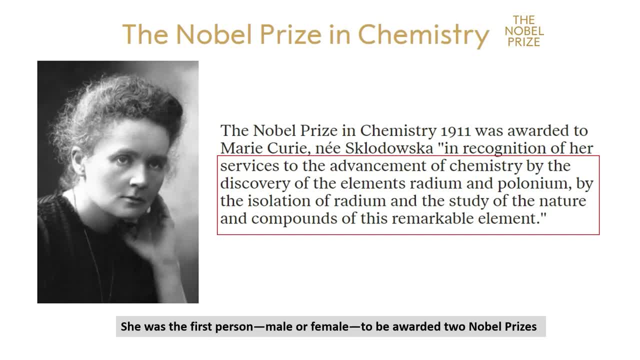 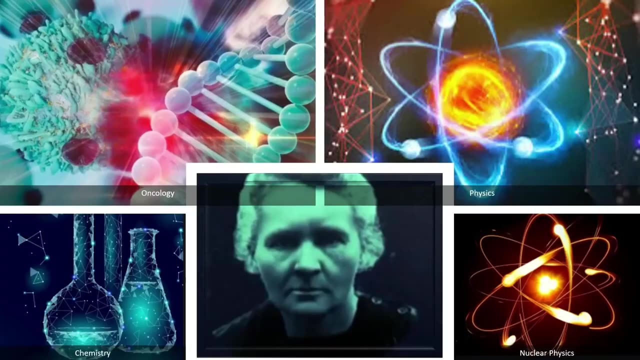 advancement of chemistry by discovery of elements radium and polonium, and also by isolation of radium and the study of the nature of and compounds of this remarkable element. and she became the first person, male or female, to be awarded two nobel prizes. so may be curious contribution to physics. 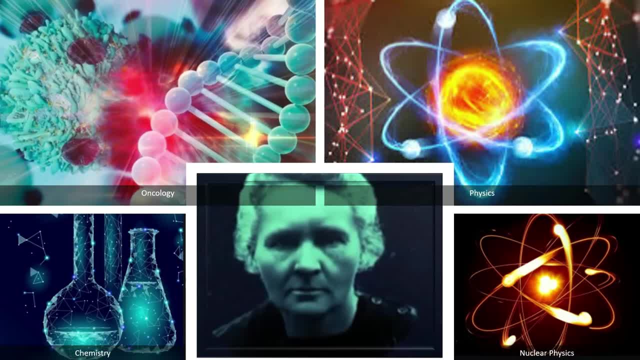 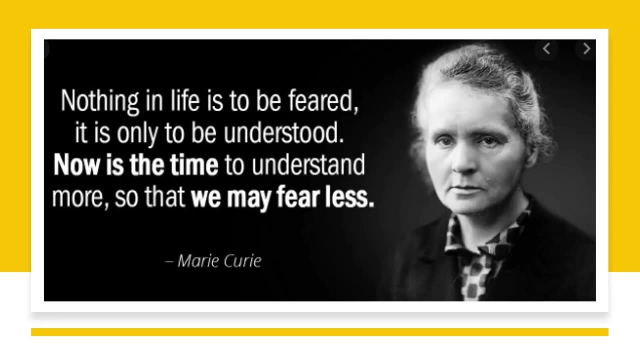 chemistry, nuclear physics and the mind-boggling discoveries and treatment opportunities in oncology is mind-boggling, is really fascinating work done by Marie Curie. and that's some motivational quotes by Marie Curie is that nothing in life is to be feared, it is only to be understood. now is it time. 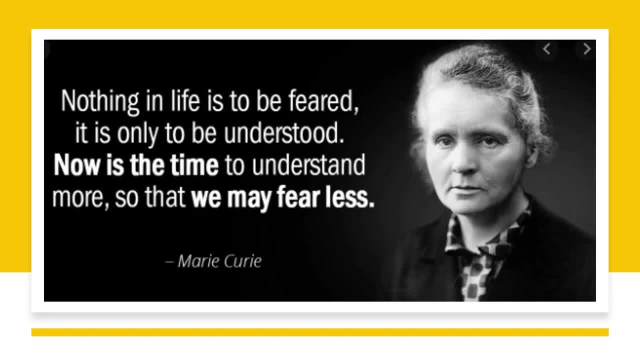 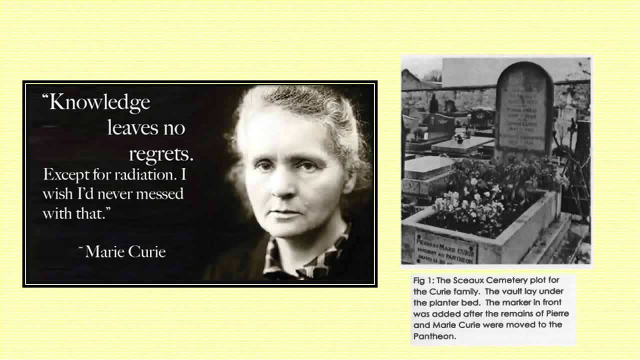 to understand more and that we may fear less. the more you understand, the less you fear, and that's one of the greatest quotation by Marie Curie- that knowledge leaves no regrets except for radiation. I wish I would never mess with that so as because whatever achievements we have or whatever path breaking, 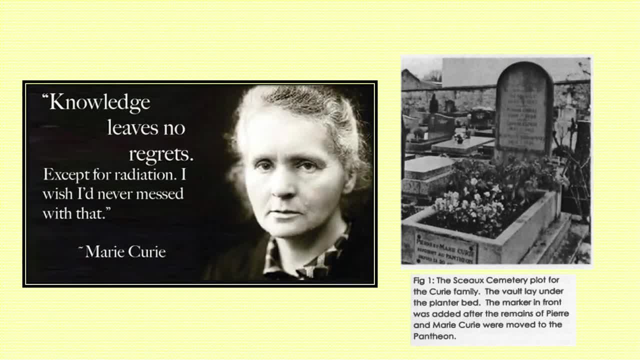 research Marie Curie did and because of which, whatever radiation physics or whatever nuclear medicine which we see, these are all because of the path breaking research laid down by Marie Curie but as a result of this, all this experimentation laid down by Marie Curie and in her family, so she was being exposed to a high radiation dose from 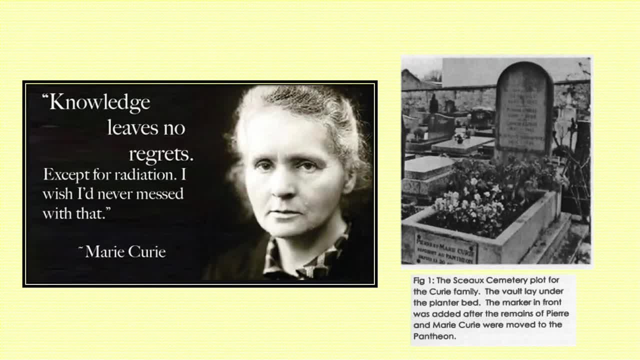 those radioactive sources and she developed a bone marrow disease and later on she died. that's why she's she says that knowledge leaves no regrets, except for radiation, explaining the lethality of radiation on the body. and that's the, the inventory plot for the Curie family and the coffin which was 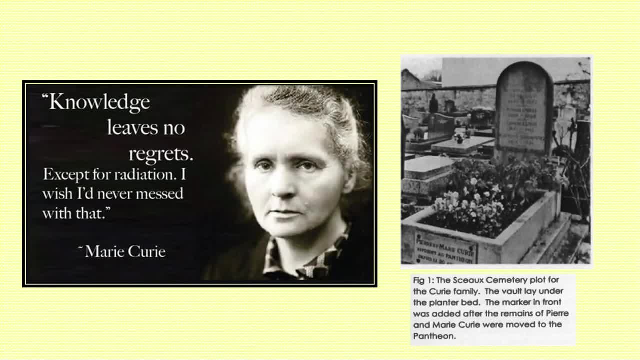 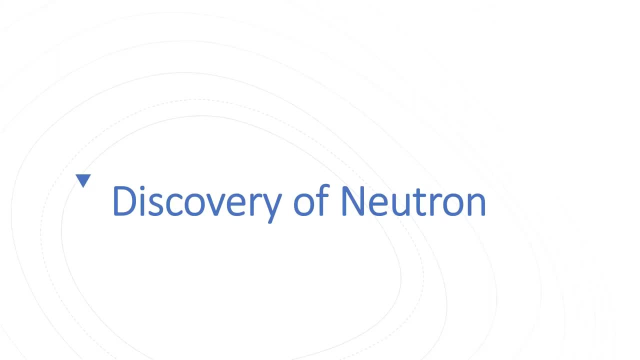 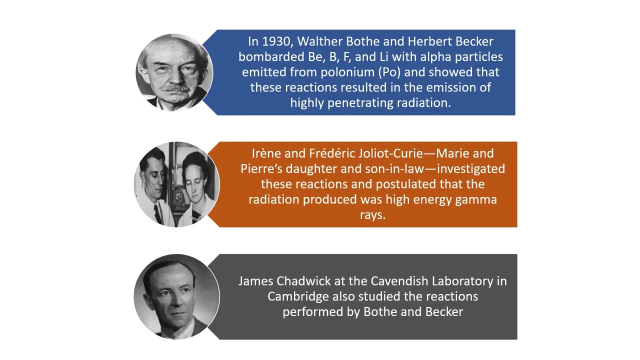 she had, she was being placed. it was, it was lead line, because her body was so radiative. so let us have a brief understanding of how the neutron was discovered. so in 1930, walter bothy and baker bombarded beryllium, boron, fluorine and lithium with alpha particles and 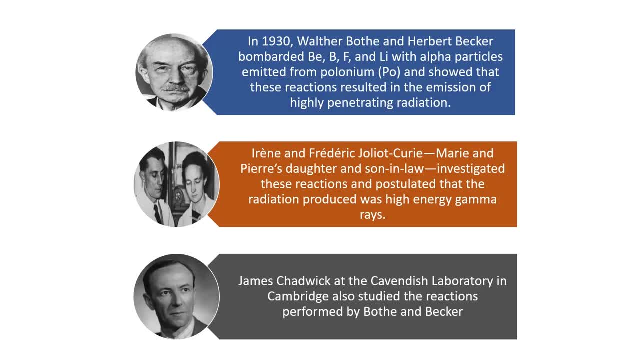 these alpha particles were emitted from polonium and it showed that after bombarding this group of elements with alpha particle, it resulted in the emission of highly penetrating radiation. and these reactions was again been uh investigated by medicare's uh daughter and her son-in-law and they postulated that uh that the radiation produced uh in this reaction. 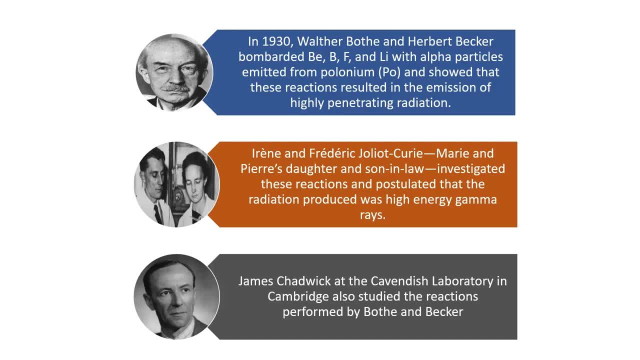 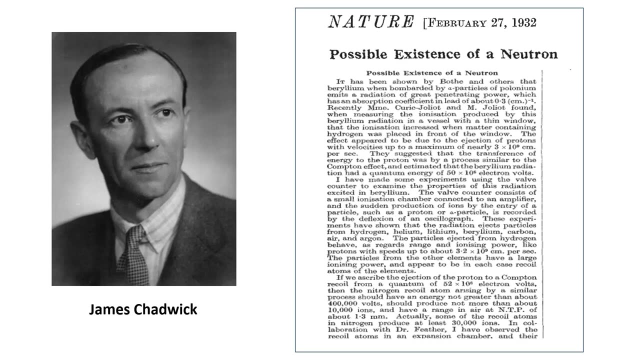 was high energy, gamma ray, photon and uh again. these reactions were again um, uh investigated by james chadwick at the cavendish lab in ambridge and uh and based on what he uh experimented with these uh reactions. so based on that he published and paper on nature on 527 uh, 1932 uh entitled as possible existence. 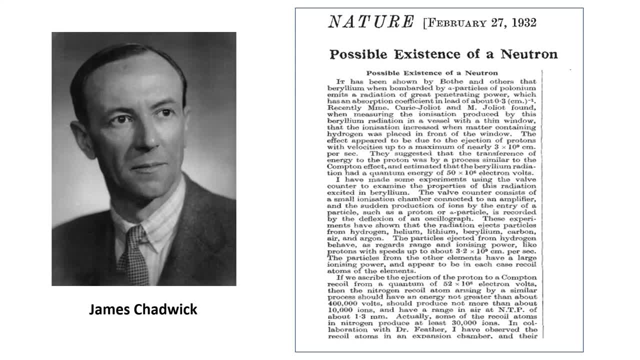 of neutron. so what it means? basically that whatever radiations was been coming out when alpha particles, uh, were being bombarded to the elements beryllium, boron, lithium or whatever- it results in the emission of neutron. so he, he are told about that, there is certain. 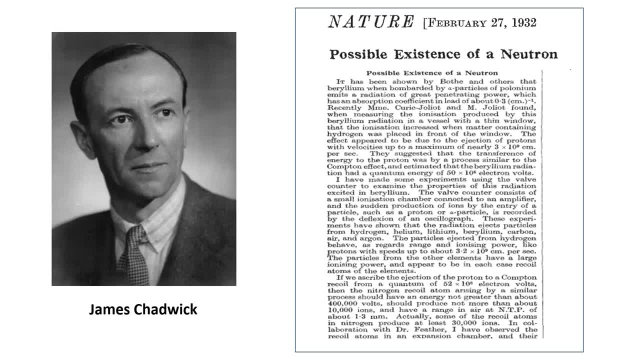 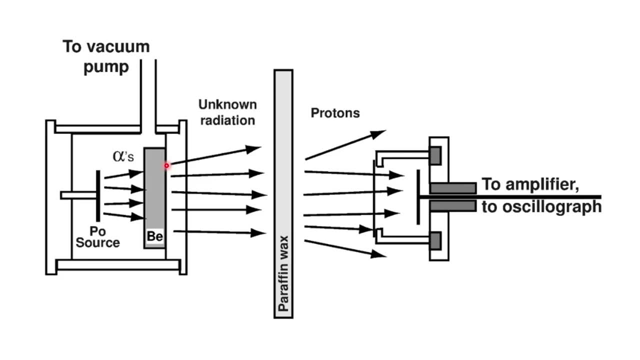 possibility that there is something we call as neutron, and that's, uh, james chedwick, who who told that it can be a neutron? and that's the experimental setup which they had. we had a source of polonium which is sending off alpha particles and it emits a radiation of great penetrating. 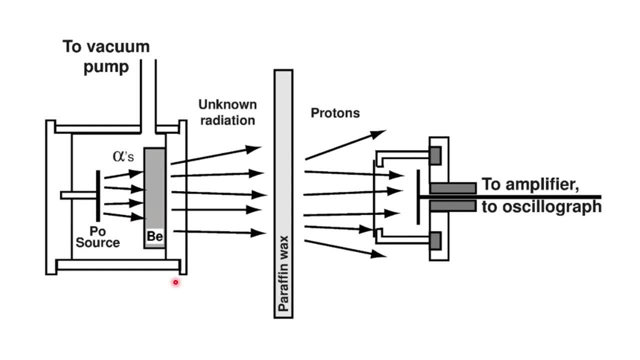 power when it hits a foil of beryllium. so something happened over here. something happened and something comes streaming out of that that could not be explained based on the current theories. and also they notice that when they placed a piece of hydrogen in the form of paraffin wax, it results in the increased amount of ionization as 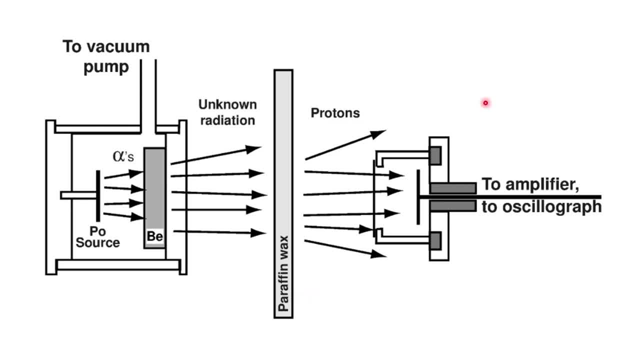 measured by the animation chamber and oscillograph, and based on that, and based on what assumption they had, or based on what estimation they had, if they told, if this unknown radiation has to be gamma ray photon, as said by irene curie and her husband, so the energy of the gamma ray photon has. 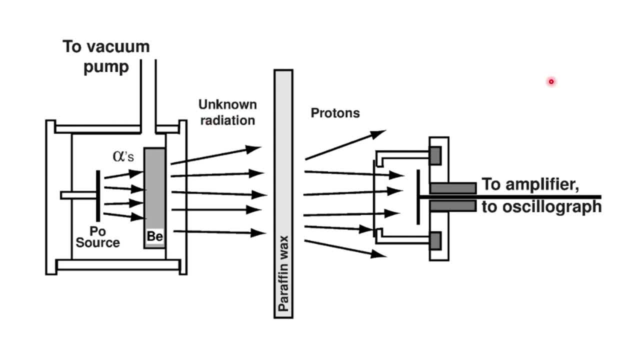 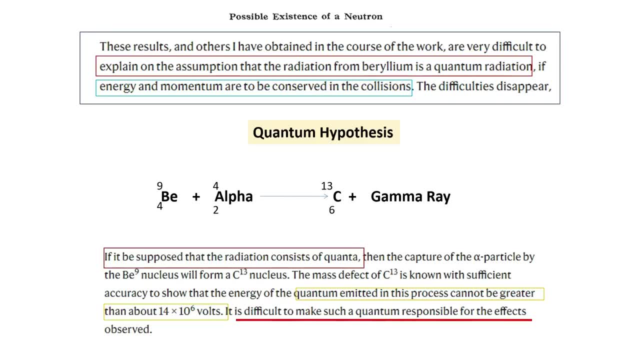 to be approximately 50- 50 mega electron volt for the amount of ionization they show over here, and if the energy of the photon is less than that, this cannot be possible, and that's the first hypothesis they had for the explanation of the same, and that is what we call is quantum hypothesis. that is the 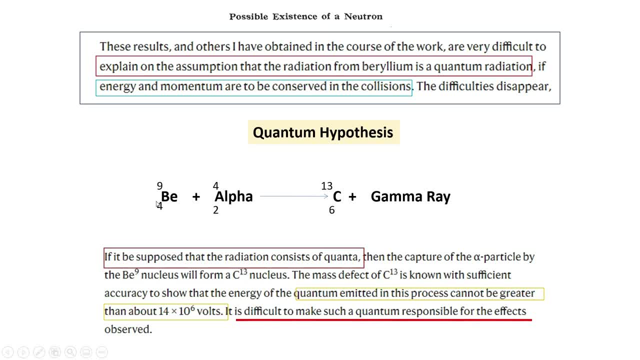 capture of alpha particle by beryllium nucleus results in production of c13 and gamma rays, and that's the gamma ray which was being emitted. uh, which is being emitted from here, but that's very difficult to explain on the on the assumption that radiation from beryllium is a quantum. 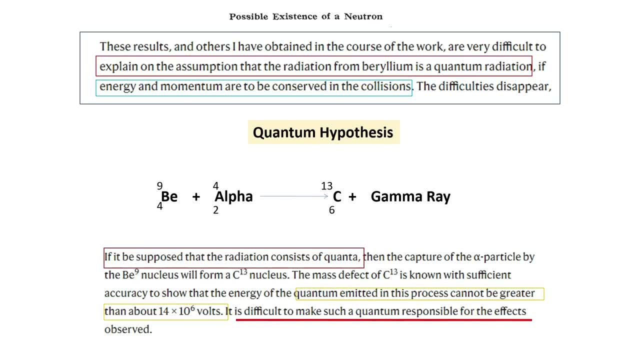 radiation, if we are trying to conserve energy and momentum, and based on the calculation which they had done, so the energy of the quantum over here cannot be greater than 14 mega electron volt, and based on the expectation of the atmosphere seen on the alpha ray photon. so if we talk about 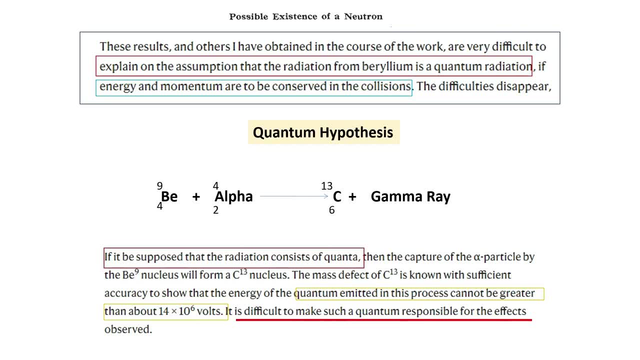 the pressure and you have just measured the rate of energy flying over there. this will provide for the ionization which you saw, uh by 14 mev of gamma ray. that amount of ionization is not possible, so we cannot be in accordance with quantum hypothesis that this cannot be a gamma day responsible for. 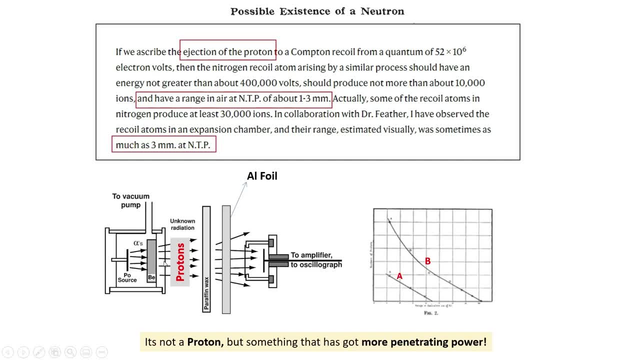 this amount of ionization that we saw. so if we ascribe the detection of proton in the process- they, like the capture of alpha particle by beryllium-9- results in emission of protons, then this proton must have a defined range in air. so what they have done, they placed an 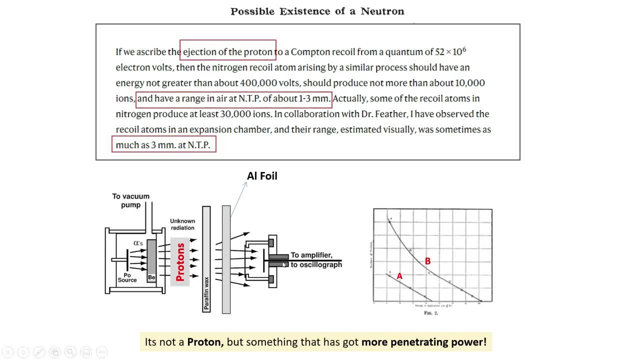 aluminum foil in between the paraffin wax and the uh, the ionization chamber and uh and the aluminum foil has defined uh thickness. so based on that they uh calculated the range of the proton. so it has to be in some somewhat like over here in about these uh range in air, but the range they 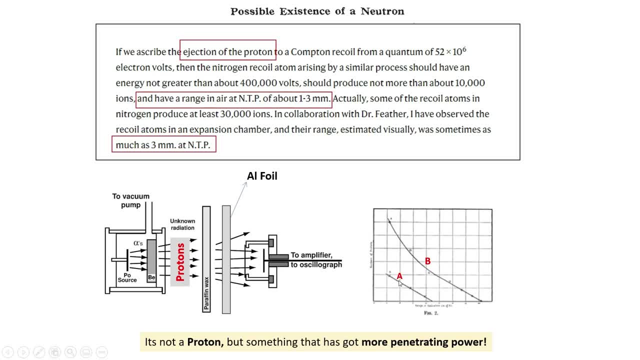 have obtained is about a three millimeter. that's, three times of the range which they actually expected. so that's very sure that that's not a proton but something else that has got more penetration power because, as these ads, because if it has to be proton, then this proton will interact with this. 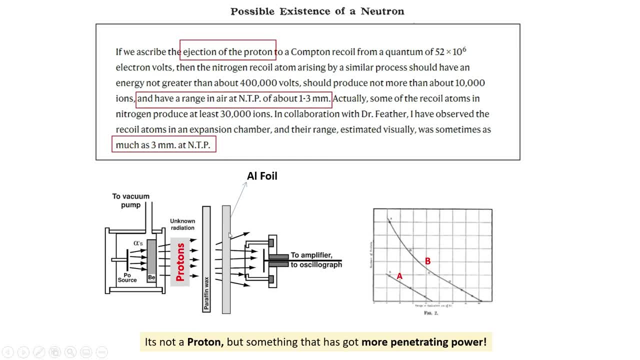 aluminum foil, because that's a charged particle, so it will interact and lose energy, so obviously the range will be. it will be lower, but as the range they obtain is quite higher, that make it very clear that's not a proton, but something that has got more penetrating power, and that's 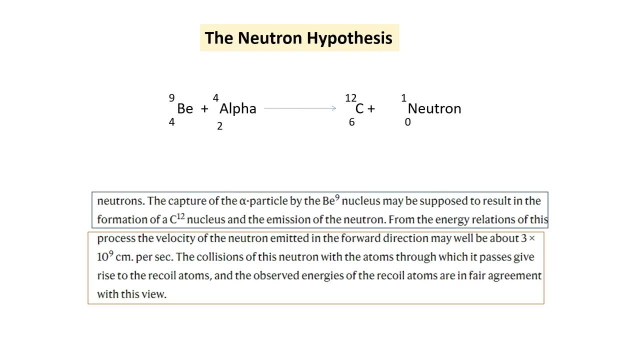 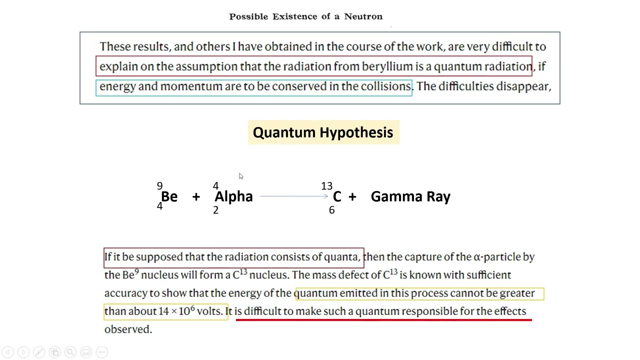 the neutron hypothesis as uh, as said by uh chadwick, that the capture of alpha particle by beryllium-9 nucleus result in emission of c12, along with neutron and uh, which the quantum hypothesis says that capture of alpha particle by beryllium-9 results in c13 and a gamma ray, but it's not c13, but 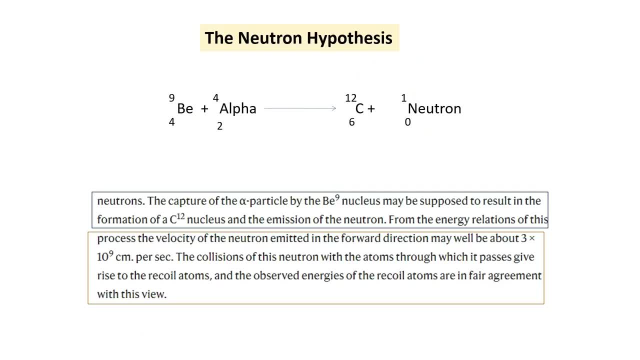 it has to be c12, along with emission of a neutron. so, and from the energy relations of this process, the velocity of the neutron emitted in the forward direction will be about three into ten to the nine centimeter per second, and the collision of this neutron will be about three. 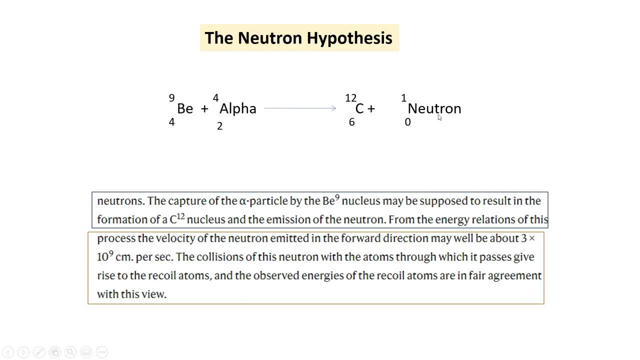 to the nine centimeter per second, and the collision of this neutron with the other atoms through which it passes give rise to recoil atoms, and the observed energies of the recoil atom are in fear. agreement, uh, with this view? that it's, uh, it's in accordance with law of conservation of. 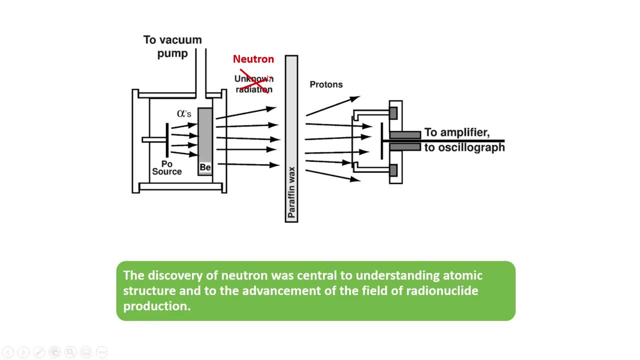 energy and momentum. so that's now we are. we are very clear now. that's nothing, but that's not gamma radiation, not proton, but these are neutrons which are being emitted from this beryllium-9 nucleus, and we all also now we all know that how uh great, uh, neutron multiplier beryllium is. so you get. 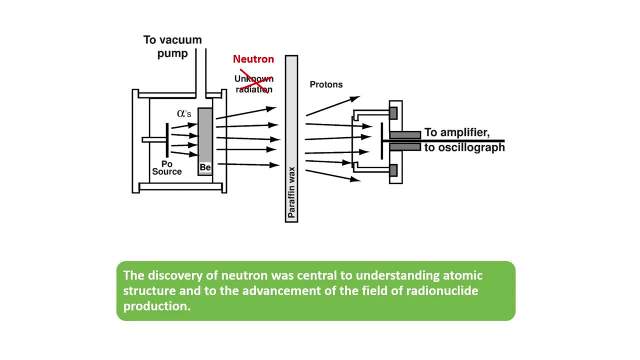 a. so you give one neutron, it gives you two neutrons back. so that's how beryllium actually works. it's a, it is an internal multiplier. oh, and that's not the uh course of understanding. so now we know that that's neutron which is being emitted from these beryllium uh nucleus. 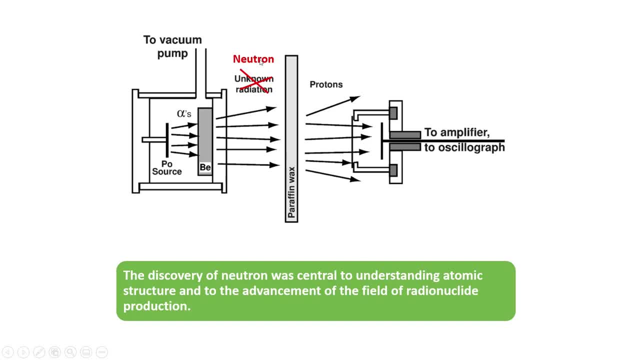 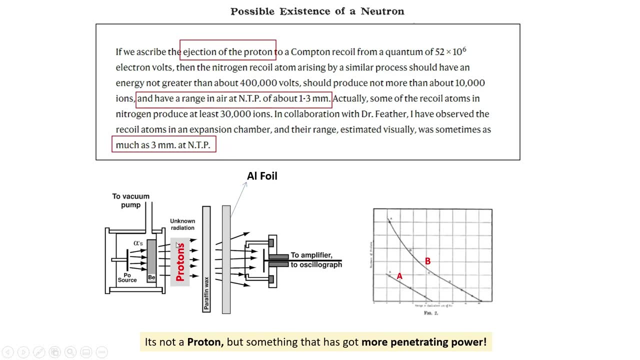 and that's not gamma radiation, not proton, and that's the main reason why it has higher range, as, because neutrons are are are neutrally charged, they don't have any charge as such, so it does not interact with the aluminum foil and that's why it has got higher range. 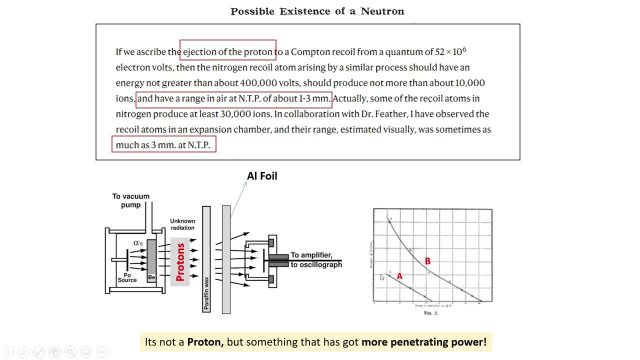 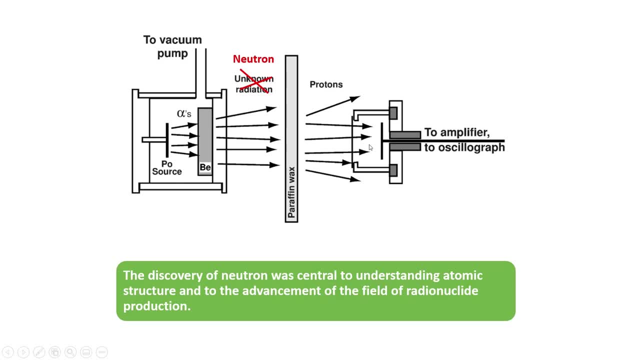 whereas protons it interacts with the foil and lose energy and thus the range is quite lesser. but that's how the neutron was being discovered and uh, and these actually opened the door for understanding the strike, understand the atomic structure and also lead the door for the reacted. 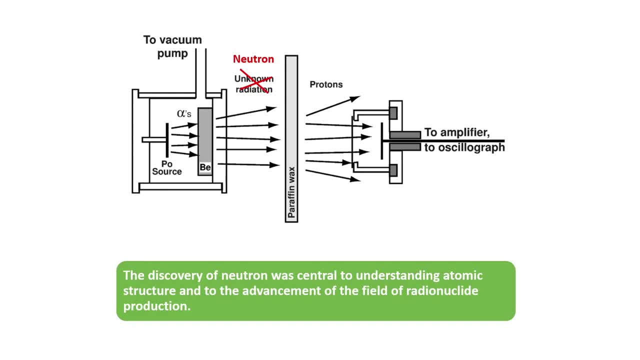 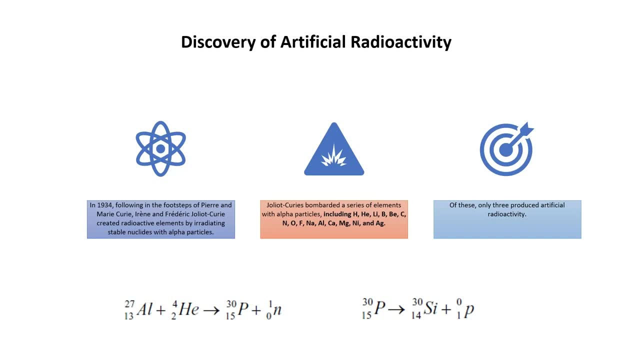 science and lead to the advancement of the radionuclide production. and that's the achievement of uh james chadwick. so the next is about the discovery of artificial radioactivity. so in 1934, following the footsteps of peary and medicuri, irene and her husband created 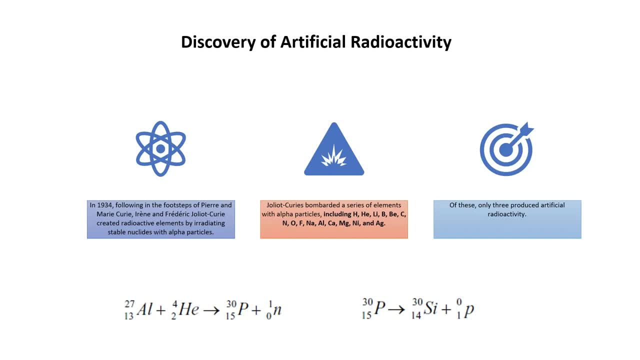 radioactive elements by irradiating stable nucleates with alpha particles. so what they have done? they have bombarded a series of elements like hydrogen, helium, lithium, beryllium, boron, carbon and these elements with alpha particles. and out of all these bombarsions, only three produced artificial radioactivity, example being aluminum when bombarded. 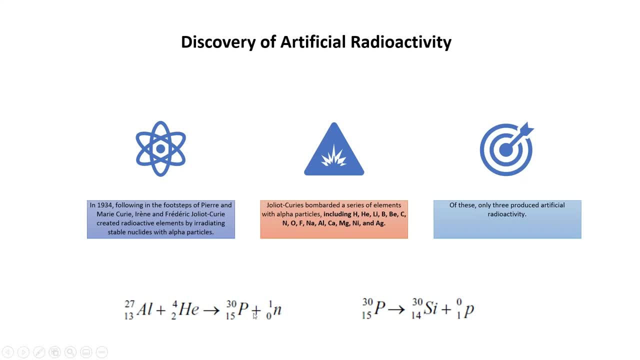 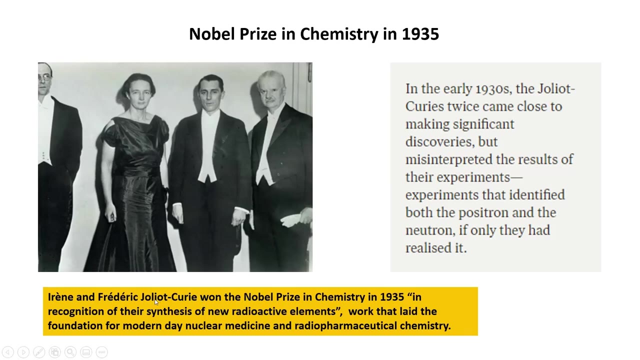 by aluminum results in production of p30 and emission of a neutron. and this p30 itself is so unstable it decays to silicon by emission of a positron. and because of this great uh discovery, uh irene and uh frederick joliot curie own nobel prize in chemistry in 1935 in recognition of their 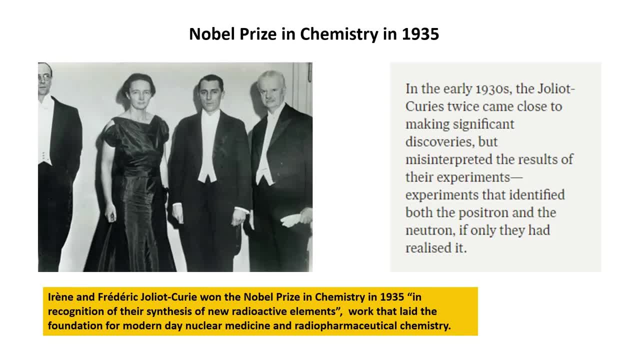 synthesis of new radioactive tracer, and these discovery laid the foundation for the modern tray and the radio pharmaceutical chemistry, because all the radio nucleates which we use for nuclear medicine are all artificially produced, for example f-18. these are being produced artificially in cyclotron. so uh but uh. irene and frederick joliot curie were very close, making two great 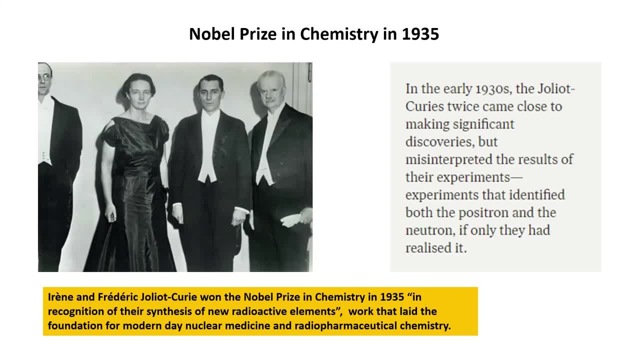 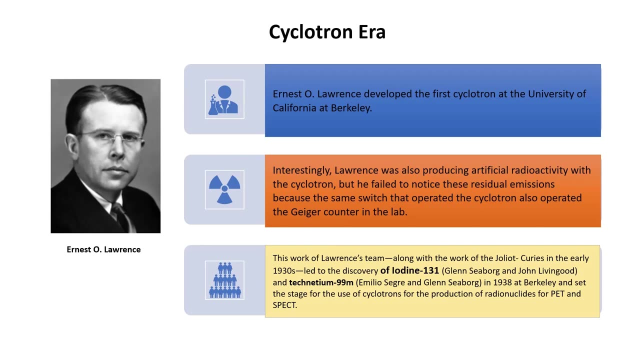 uh discoveries like uh for discovery of positron and neutron. but because of their misinterpretation they were very close to it, so but they could not make it out. but still they got nobel prize. so the next is on the cyclotron era. so arnst lawrence developed the first cyclotron at 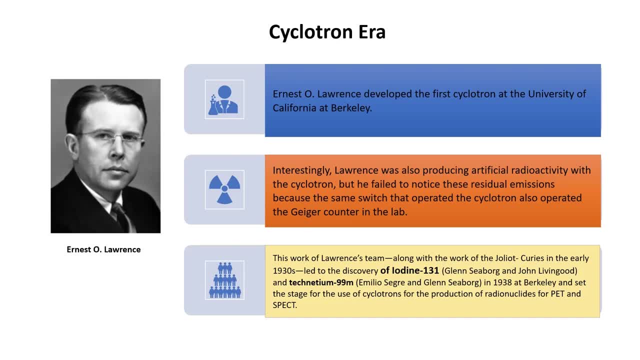 the university of california at berkeley. uh, interestingly, lawrence was also producing artificial radioactivity, like what irene curie did, but he failed to notice these residual emission because the same switch that operated the cyclotron also operated the giger counter in the lab, and that's why he failed to notice the residual emission. and 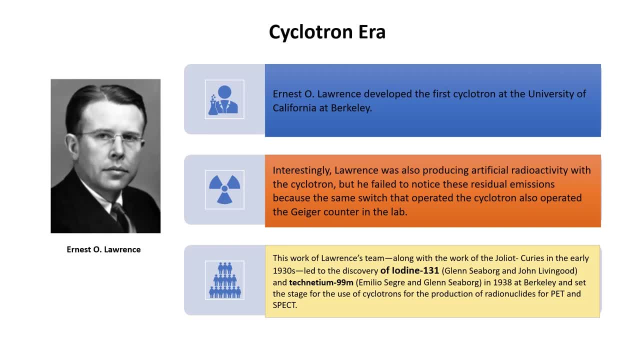 these are the results of the research that we are going to show you in the next slide. so the next is on the cyclotron era. so arnst lawrence developed the first cyclotron at the university of california, and these work of lawrence team, along with the work of joliot 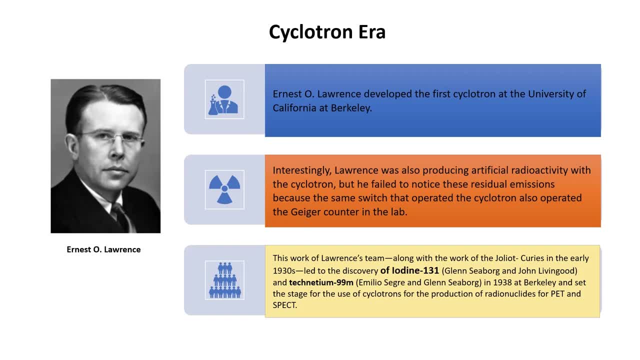 curies in the early 1930s led to the discovery of iodine-131 by glenn seaborg and john livinggood and technetium by these people in 1938 at berkeley, and set the stage for the use of cyclotron for the 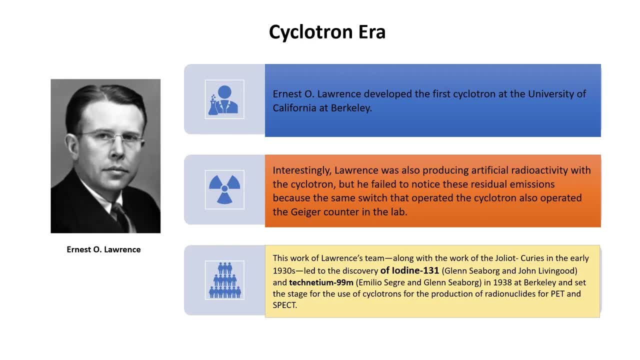 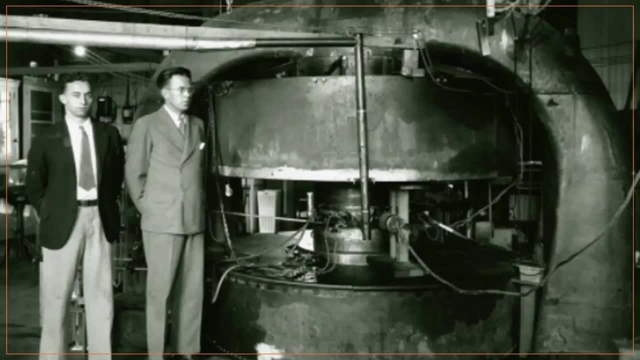 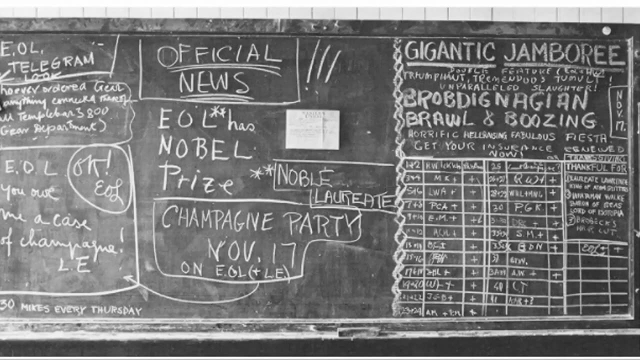 production of radio nucleates for pet and spect. that's a great milestone achieved by this group of people. and that's arnst lawrence with his developed cyclotron, and that's the image of patent as filed by uh your lawrence and that's the greatest news that uh, he had that. 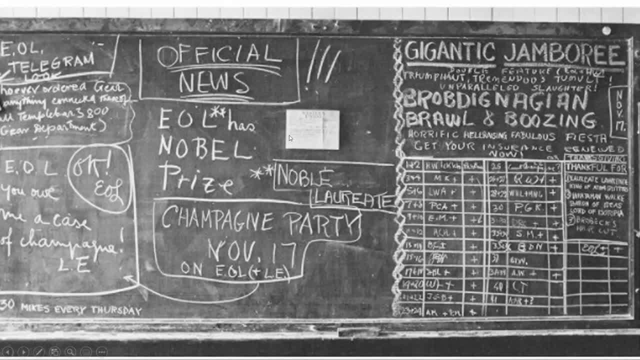 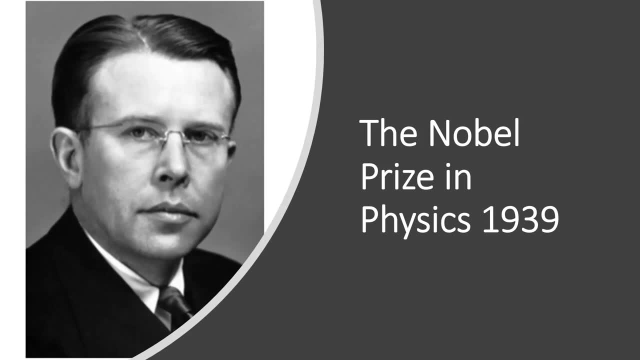 he has owned the nobel prize. so ernst, or lawrence, has the nobel prize, nobel laureate and champagne party november 17.. and because of his greatest uh development of the cyclotron, he was being awarded nobel prize in physics. so that's the greatest quotation which 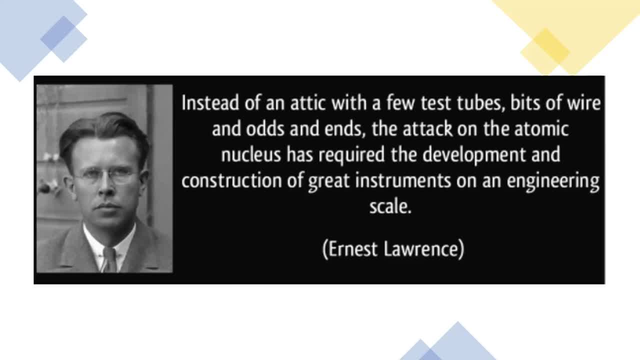 i can tell you about, instead of an attic with a few test tube, bits of wear and odds and ends. the attack on atomic простоdoor was not simple. the attack on atomic simply has required the development and construction of a great instrument on an engineering scale. so it might. 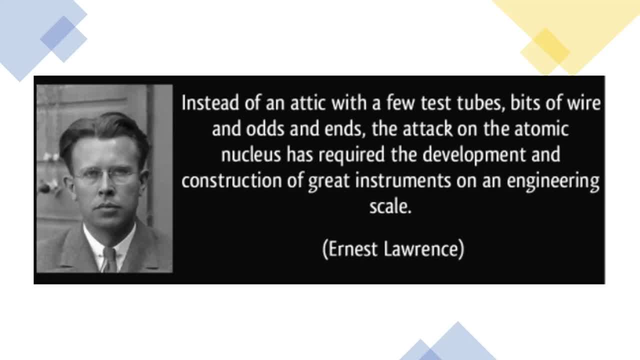 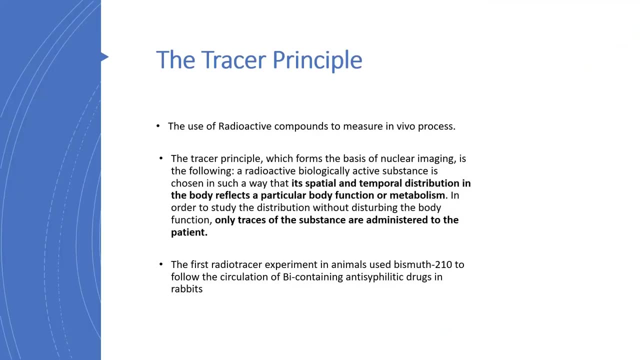 look very simple, but cons about attacking on the simplest atom was not a simple. attacking on the atomic Oğlum has required the development and construction of a great instrument on an engineering scale. of discussion today is on the tracer principle. so what is all about the tracer principle? so the use 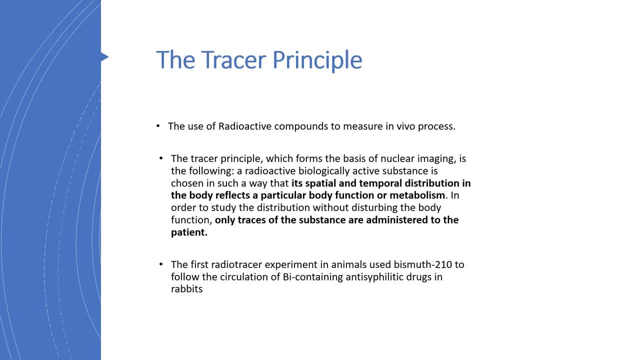 of radioactive compounds to measure in vivo process is what we call as the tracer principle. so the tracer principle, which forms the basis of nuclear imaging, is the following: so what we do is that a radioactive, biologically active substance is chosen in such a way that its spatial and 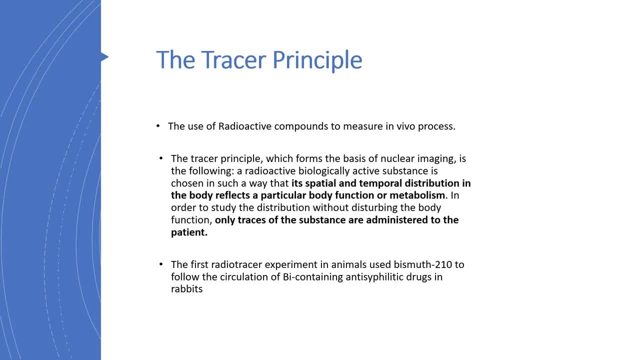 temporal distribution in the body reflects a particular body function or metabolism. so in order to study the distribution without disturbing the body function, only traces of the substance are administered to the body of the patient and that's why we call as tracer, because only some, because only traces of the of the molecule are being administered and these studies were being first. 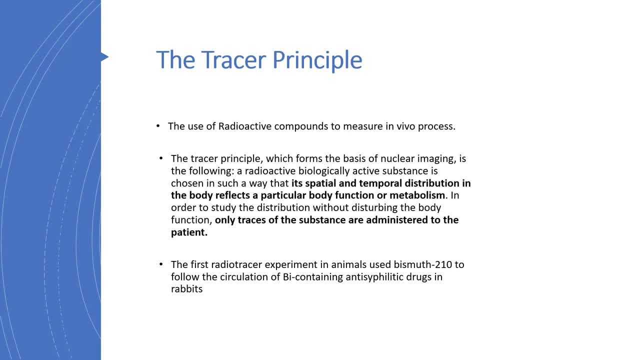 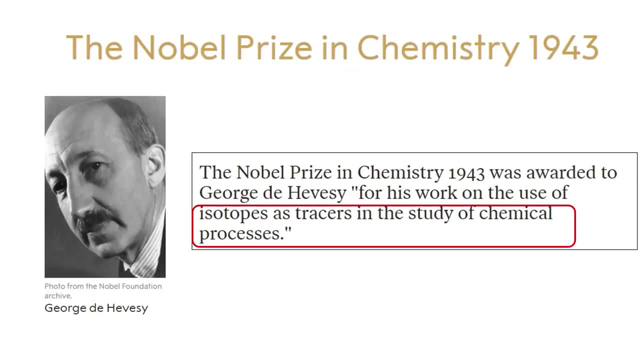 uh done in experiment, uh um, and they used bismuth 210 to follow the circulation of bismuth 210 to follow the circulation of bismuth 210 to follow the circulation of bismuth containing anti-siphonic drugs in rabbits. and because of this greatest uh work. 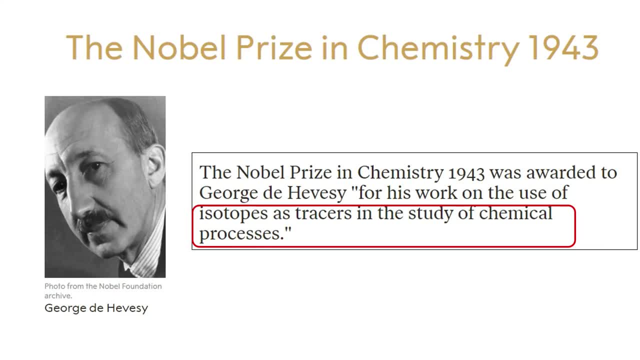 george d havesi was being awarded a nobel prize and being called as the father of nuclear medicine. so and this award was being given to george d havesi and the nobel prize in chemistry 1943 for his work on the use of isotopes as tracer in the study of chemical process. 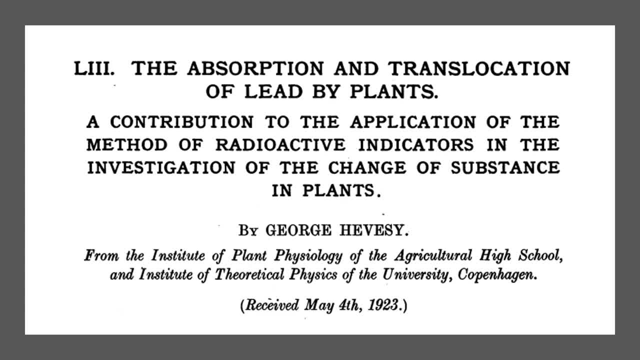 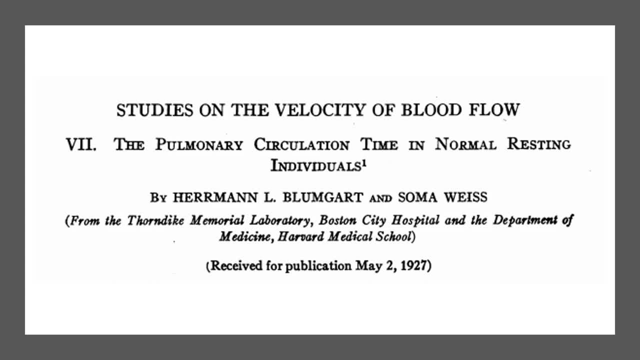 and that's some of the work done by george havesi, and that's on the absorption and translocation of lead by plants and that's the initial studies on the velocity of blood flow using the radio tracers. and now moving forward to the discovery and the 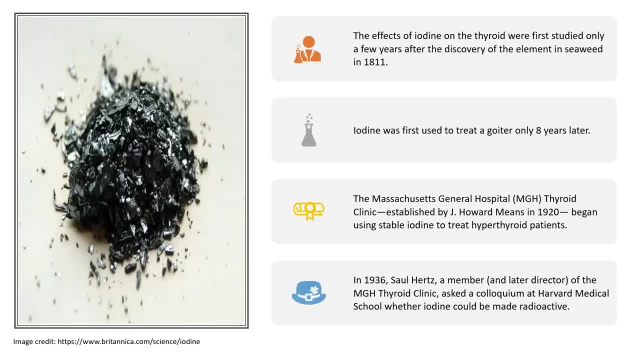 use of radionuclides of iodine. the effect of iodine on the thyroid were first studied only a few years after the discovery of iodine in seaweed, and in the initial days iodine was used to treat greater and uh. the mgh thyroid clinic established by jay howard means 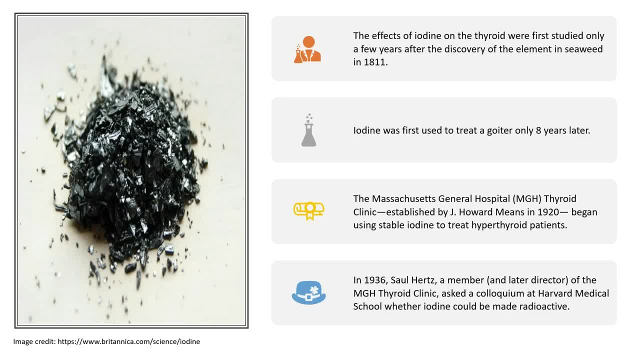 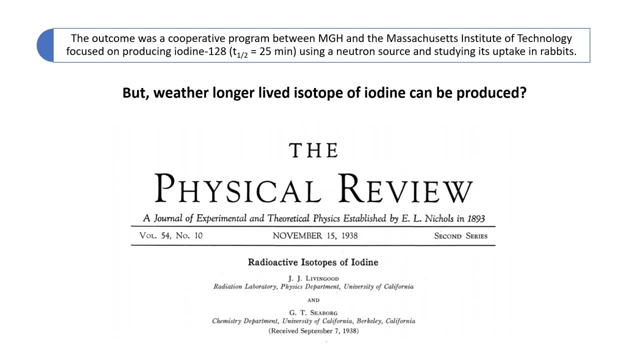 stable iodine to treat hyperthyroid patients. and in 1936 saul huts, a member of the mgh thyroid clinic who later became the director of the same, asked a colloquium at harvard medical school whether iodine can be made radioactive or not. so the outcome of was a cooperative program between mgh and the mit. 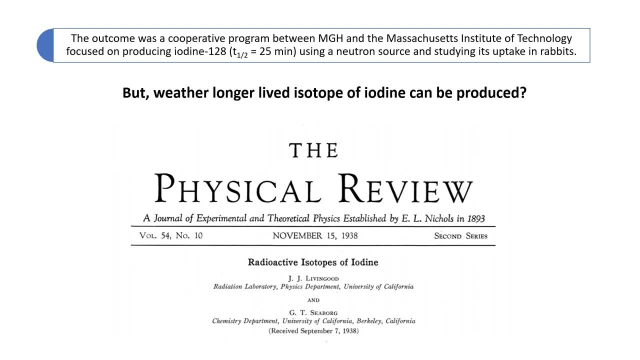 which focused on producing iodine-128 using a neutron source and studying its uptake and rapids. iodine-125 has a smaller half-life of about 25 minutes. now the next question was whether a long-lived isotope of iodine can be produced or not, and to that, to that question answer was with: 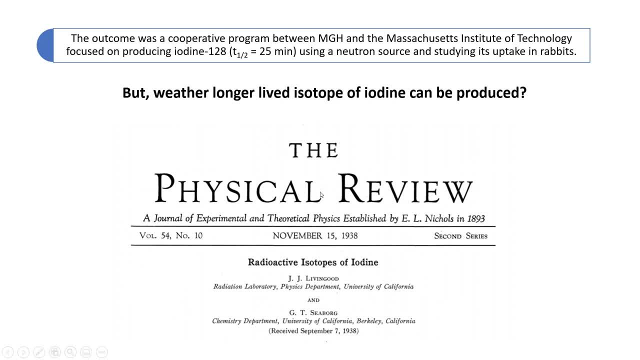 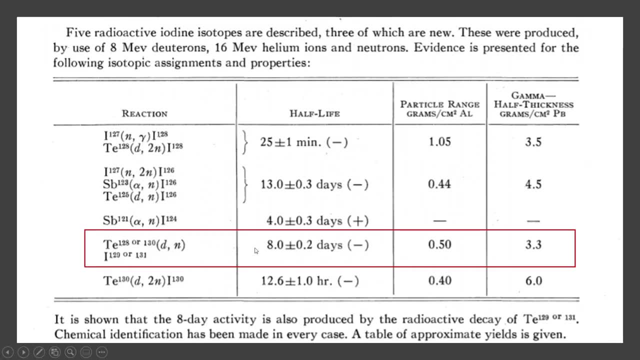 from jj living good that he published an article on the physical review named as a radioactive isotope of iodine, in which he mentioned about five radioactive iodine isotopes, and three of which are new. so these were produced by using 8 mav, deuterons, 16 mv, helium ions and neutrons, and these are this: 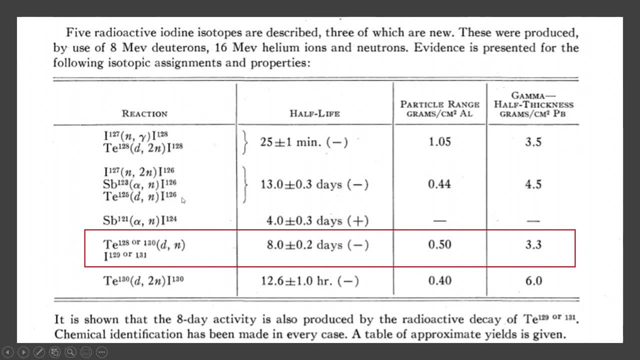 group of uh isotope, that being that are being prepared for from the same: iron 128, iron 126, iron 124, iron 130 or 131 and again 130.. so, out of these, uh, the uh, the interest of us in uh, of interest of our, is in iron 130, which has an half-life of eight days and which was produced. 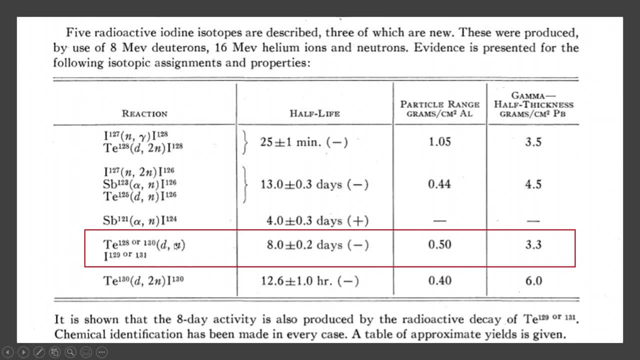 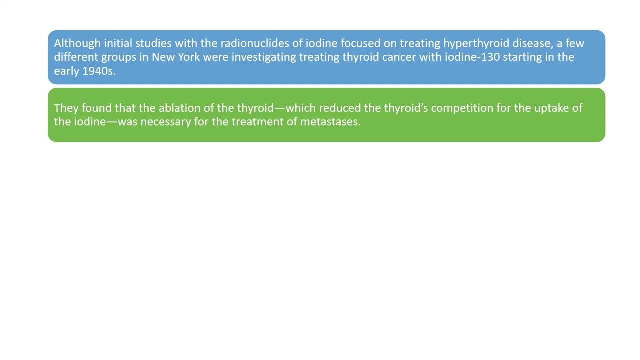 uh or 130 by deuterons and lead to the production of iodine-129 or iodine-130, so a 131. so that's about the initial uh, uh, initial discoveries of iron 31 through this process and uh, although the initial studies with the radionuclides of iodine focused. 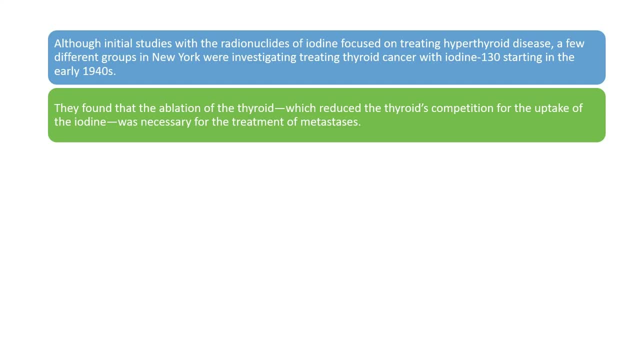 on treating hypertheroid cases- uh hypertheroid diseases. so the initial uh studies were based on the treating hypertheroid diseases. but a few different groups in new york were investigating treating thyroid cancer, also with arden 130, and what they found is that uh is very important that 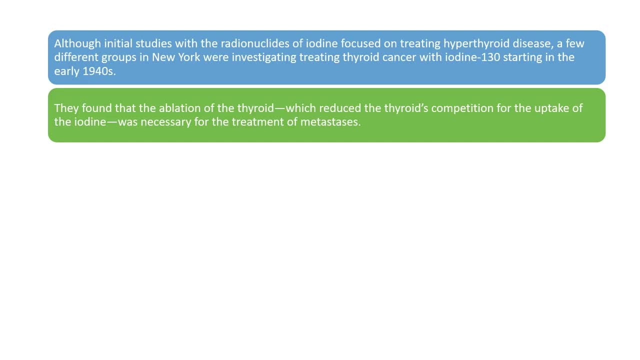 the abolition of thyroid, which reduced thyroid competition for uptick of iodine, was very important for treatment of metastasis and that's one of the initial studies on the treatment of thyroid carcinoma with radioactive iodine-131. and because of these great, uh, uh, great innovations, 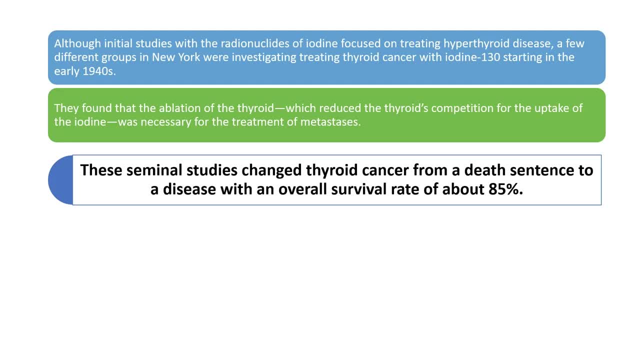 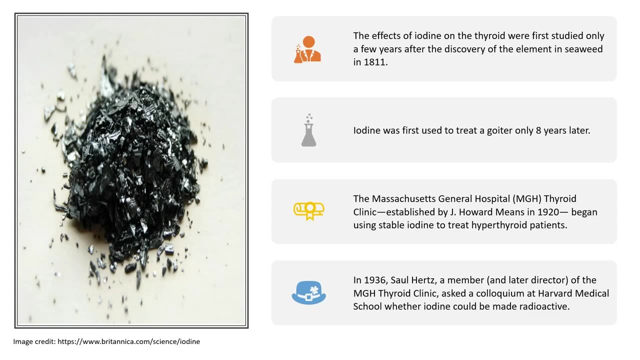 and the initial seminal studies. it changed the thyroid cancer from being a death sentence to a disease with an overall survival rate of 85 percentage. now we can see how questioning is very important. that, like from the initial time, we have been using a normal iodine for treating quitter. then we 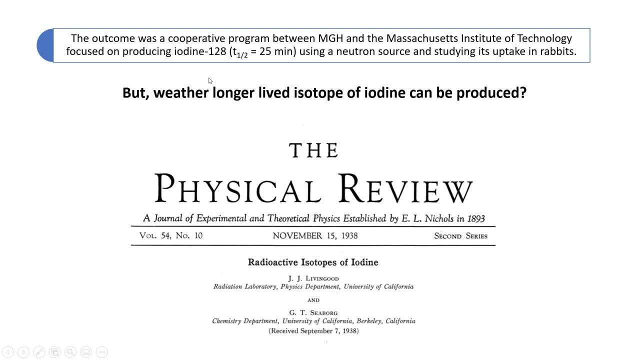 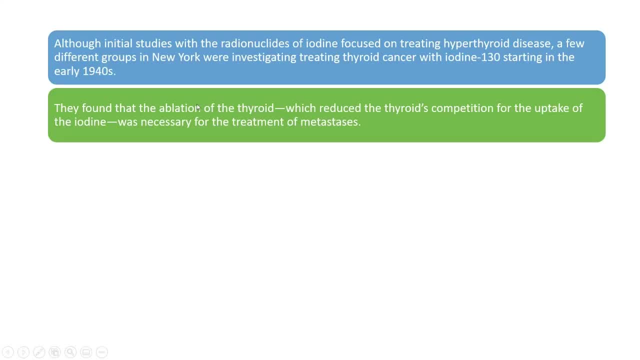 asked about whether uh x asked about radioactive iodine, then we asked about longer lived iodine, and then we got to know about iodine-131, and then studies, and studies, and studies. and then we've got to know about treatment of thyroid carcinoma about with radioactive iodine. so those studies are very 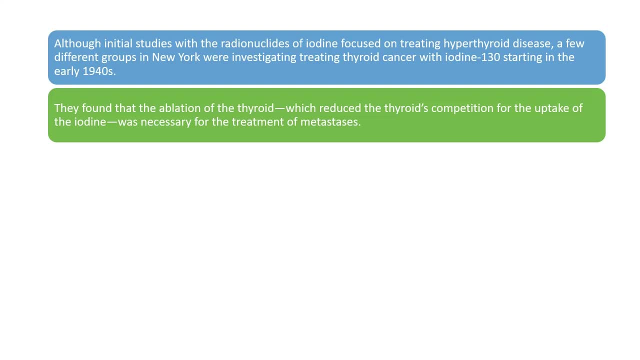 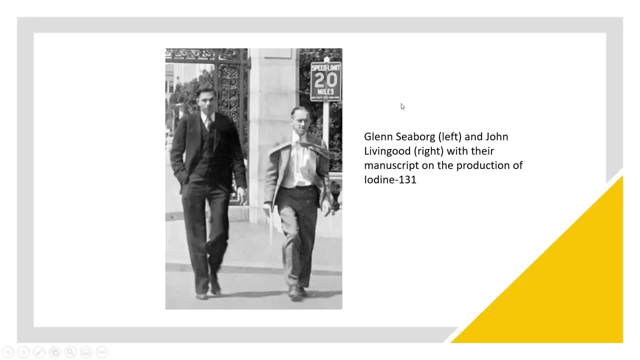 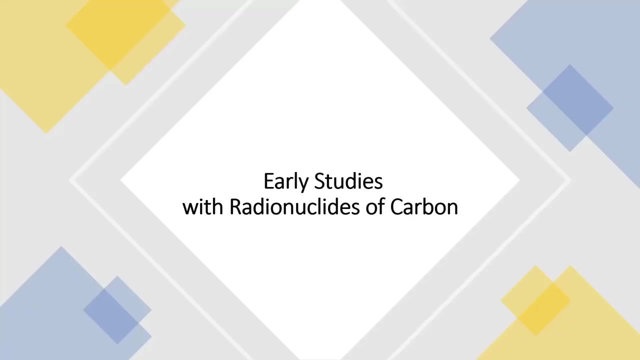 important and, apart from this, what is what is more important is about asking question on the prevailing situation is also very important. so that's uh, glenn zeebock and john living good, uh, with their manuscript for the production of iodine-131, and now moving forward to the 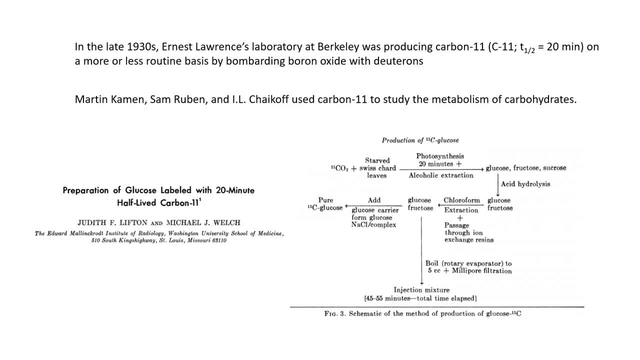 early studies with radio uh, with radionuclides of carbon. so in the late 1930s, ernst lawrence, a lab at berkeley, was producing carbon eleven and this carbon eleven whose has a very shorter half time of 20 minutes, so it was being made by bombarding carbon dioxide with deuterons. 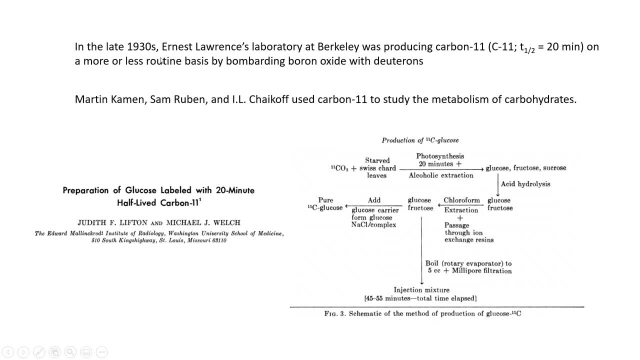 and this group of people used carbon eleven to study metabolism of carbohydrates and that's the initial paper published by some other people, uh on preparation of glucose level with c-11. but now we now let's see how beautifully they have produced uh c-11 level glucose and uh the 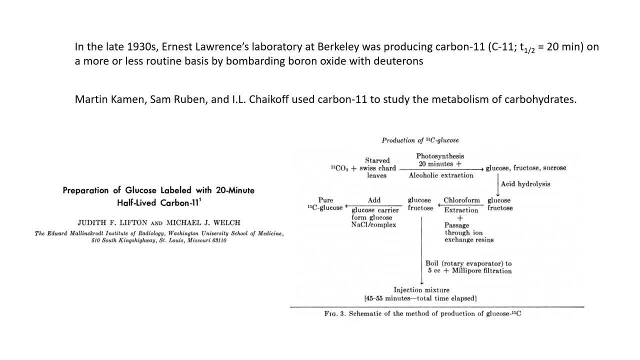 to the used radioactive uh, co2, uh radio, c11, co2 gas and they are, and again they gave it to the starved uh sweet chart leaves and through photosynthesis and through this uh for this process, they produced pure c11 level glucose. that's the creativity we can understand by using 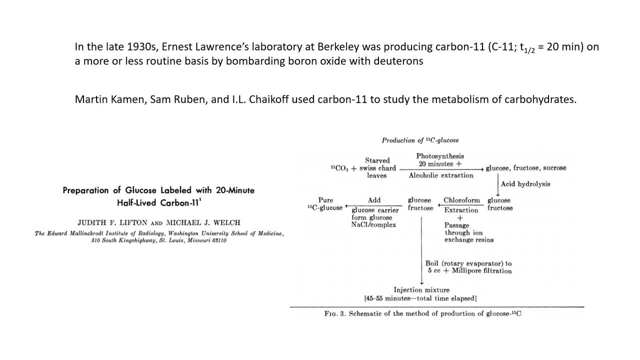 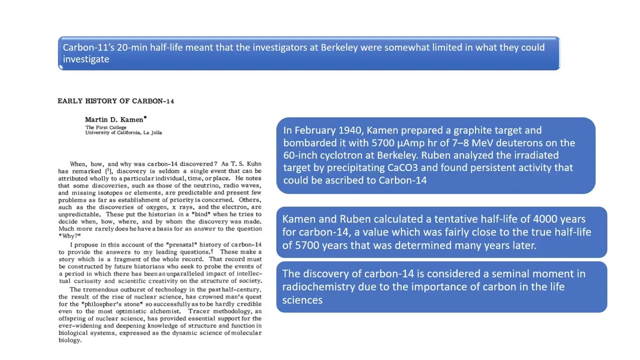 plant as a generator for production of glucose. so that's the creativity of these people. so today we are using chemistry modules for production of ftg, but at that time they are using plants to produce uh c11 glucose and with this glucose they studied uh multiple things, but uh the c11 glucose. 20. 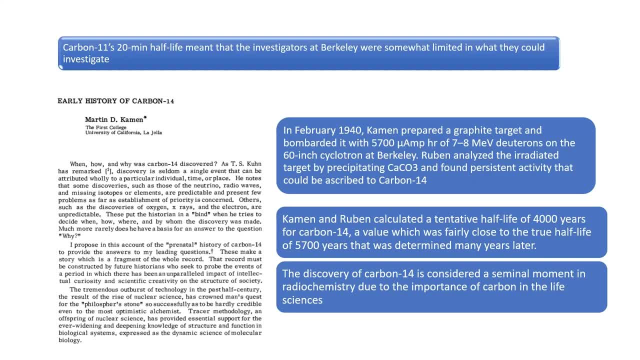 minute half-life, uh means that the investigations at berkeley were somewhat limited because, uh, it has a very half-life, very short half-life. so in faf 1940, cameron prepared a graphite target and bombarded with it these, uh, this configuration of deuterons, on on these configuration of. 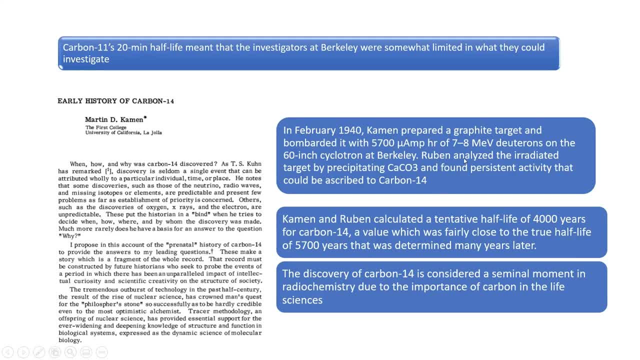 deuterons at berkeley and uh, what they got is. uh is, what they got is a c14 and that's the initial paper published by martin de camen for the early history of c14. and this discovery of c14 is considered a very seminal moment in radiochemistry because, due to its importance in uh, importance of 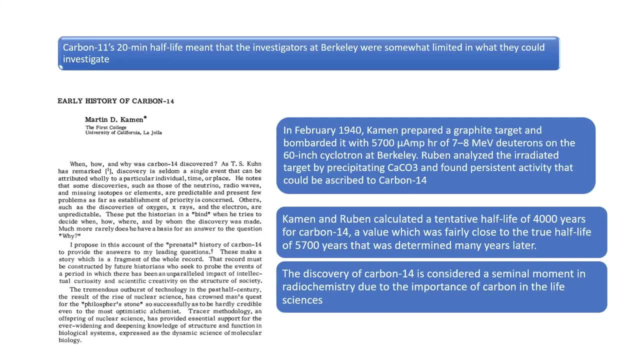 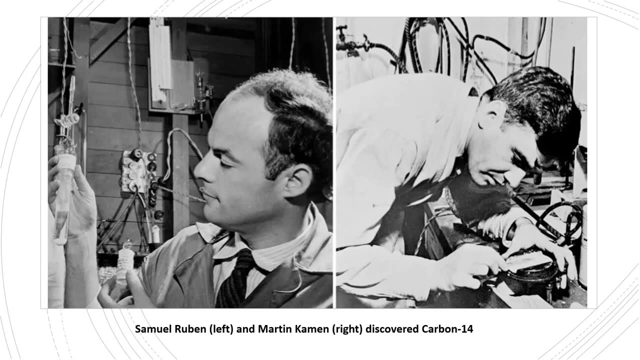 carbon in the life sciences, like c14 dating, which, what you, what we do today, these days, is all based on c14 and that's the milestone achieved by um, by uh cameron and berkeley, and that's what they got ruben for discovering c14, and that's uh. samuel and ruben and martin camen who discovered c14. 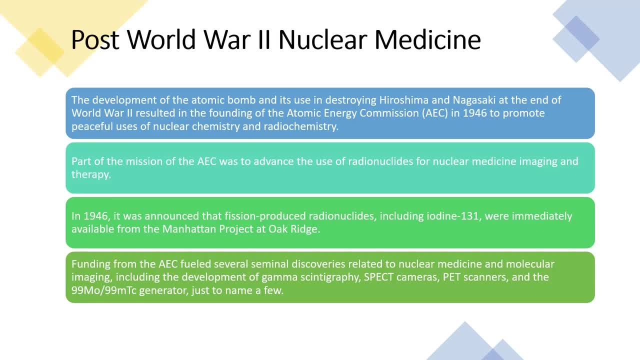 now moving forward to the post world war ii nuclear medicine. so development of atomic bomb and its use in destroying hiroshima and nagasaki at the end of world war ii resulted in foundation of the atomic energy commission in 1946 to promote peaceful use of nuclear chemistry and radio. 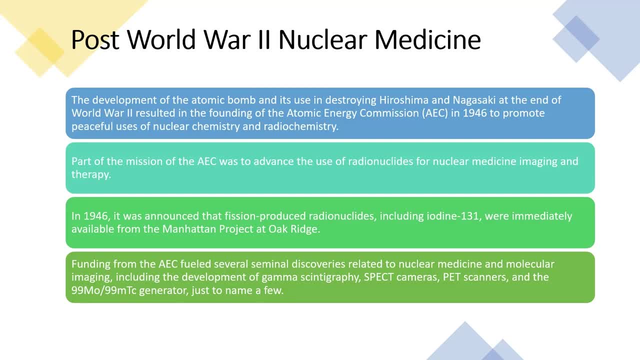 chemistry. so, and part of the mission of this aec was to use the nuclear bomb. as a nuclear bomb, the radionuclides of car, of uh, was to use uh and part of this mission of this aec was to advance the use of radionuclides for use in nuclear medicine, imaging and therapy. and in 1946, 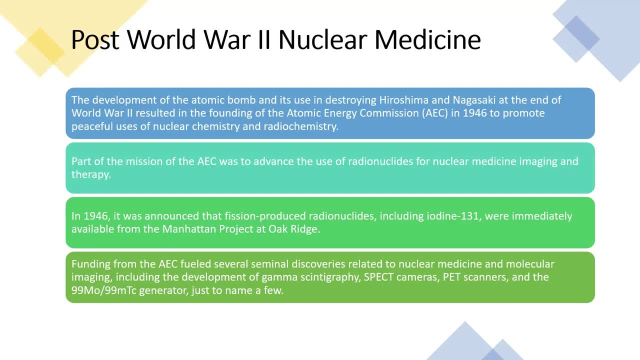 uh. it was announced that the fission produced radionuclides including iodine-131 was immediately available from the manhattan project at oak ridge, and these funding from this atomic energy commission actually fueled several seminal discoveries in nuclear medicine and molecular imaging, including development of gamma centigraphic cameras. 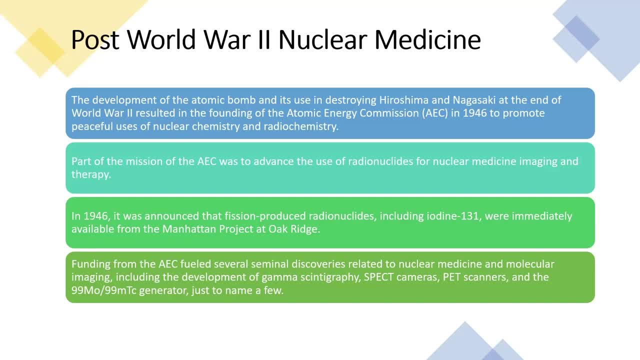 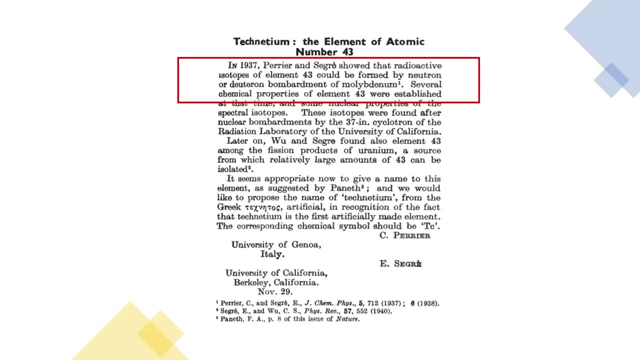 spec cameras, spat cameras and the moly generators are just few names, and these aec funded several milestone projects, which has led to today's nuclear medicine now moving forward to technetium generators and technician label pharmaceuticals. that's how technetium came into picture, by 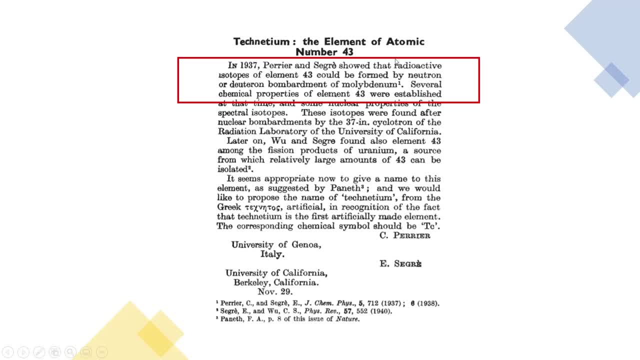 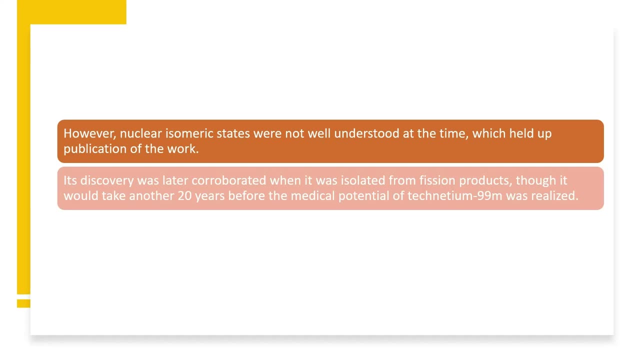 perrier and and segre showed that bombarding neutron or deuteron or to molecular medical lead to production of technetium. so but these are the was not clear because the nuclear isomeric states were not well understood at that time and which held up the publication of the work, but its discovery was later, was 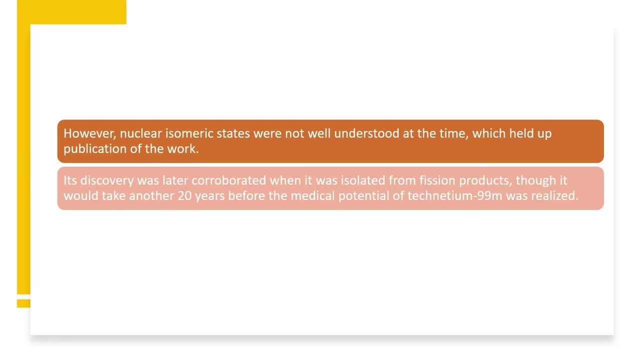 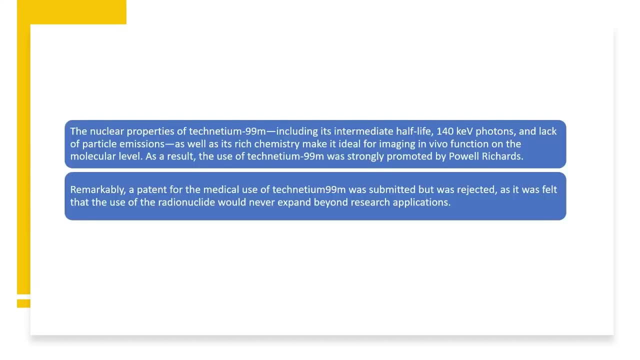 later collaborated um when it was isolated from fission products, though, it would take another 20 years before the medical potential of recognition was being realized. so, uh, the most important things about magnesium is about the properties which it uh, which it uh it has, including its half life, including its energy of photon: 140 kilo electron volt. 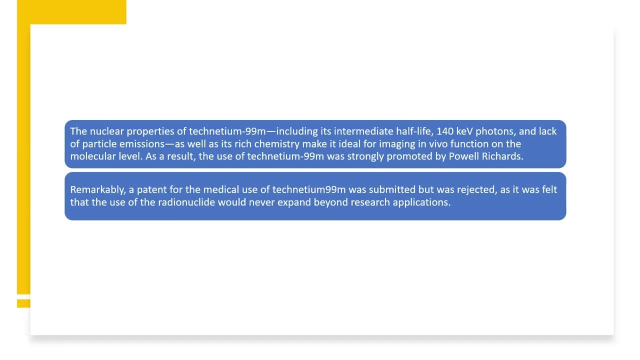 its lack of particle emission and its rich chemistry, it makes it ideal for imaging the in vivo functions of the at the molecular level. and as a result of its great properties, uh, the use of technetium was was strongly promoted by powell richards and, remarkably, a patent was also. 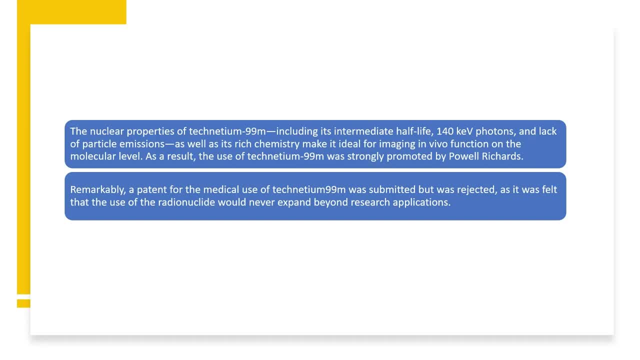 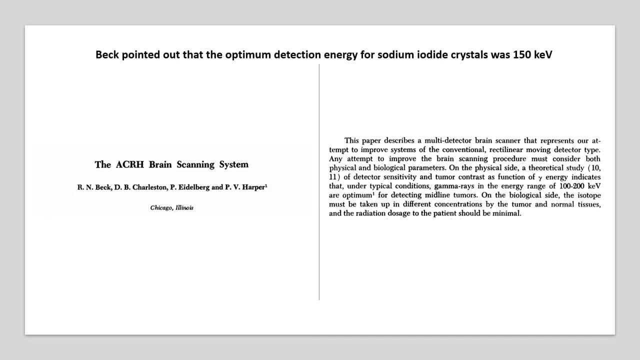 filed for the use for the medical use of technetium, but it was rejected because it was felt at the time that the use of radonuclide would never expand beyond research applications. but it all changed when Beck pointed out the optimum detection energy for sodium iron crystals was 150 kilo electron volt and 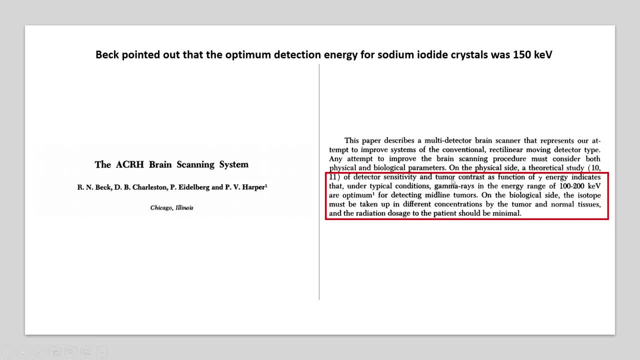 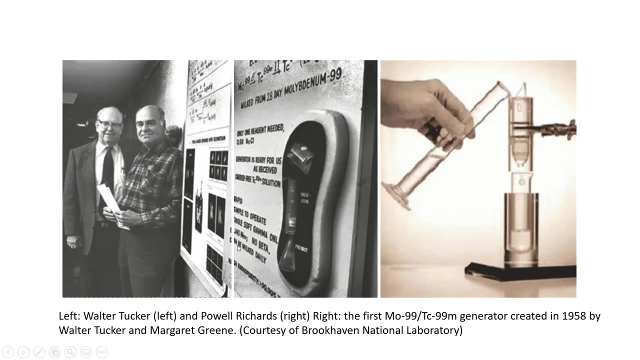 that's from here. that for the good tumor contrast as a function of gamma in energy indicates that under typical conditions gamma rays in the energy range of 100 to 200 keV are optimum for for detecting midline tumors. and it changed the whole new world. and that's Walter and Powell Richards and that's the. 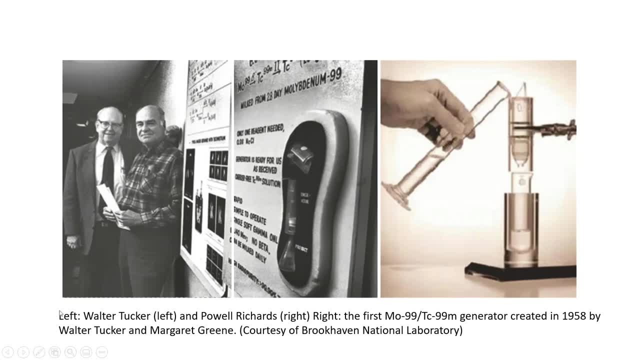 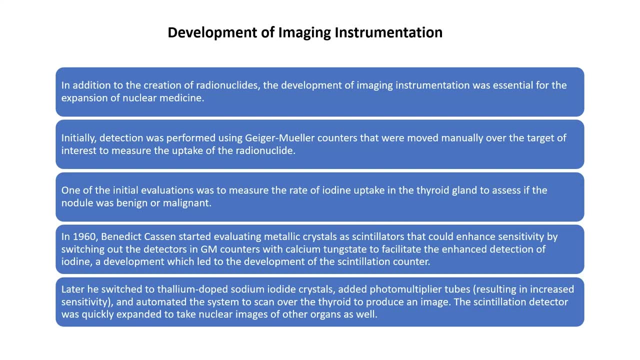 first moly generator, created in 1958 by by this group of people, and now moving forward to development of imaging instrumentation. so, in addition to the creation of radonuclide- because now what? whatever you have seen- we have created radonuclides, but development of radonuclides is not the end of the world. so, in addition to the creation of radonuclide- because now what? whatever you have seen, we have created radonuclides, but development of radonuclide is not the end of the world. 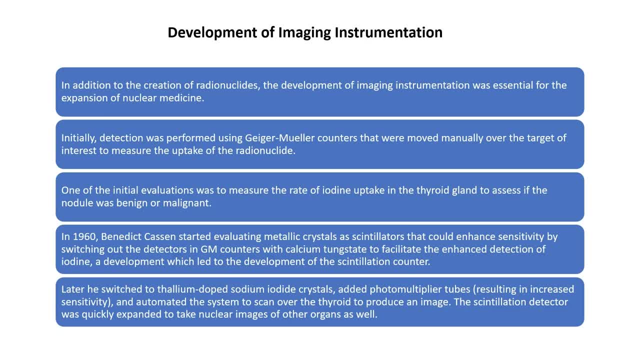 of radonuclides is incomplete without the development of imaging instrument because that will give you how your pharmaceutical has distributed inside the body. so the development of imaging instruments was very critical for the expansion of nuclear medicine and the initial detection was performed using GM counter and that were moved manually over the target of interest to measure. 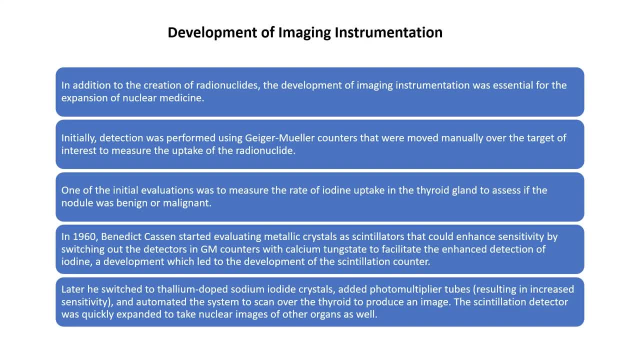 the uptick of radonuclide, and one of the initial evaluations was to measure the rate of iron uptick and in the in the thyroid gland and to assess if the rate of iron uptick and in the in the thyroid gland and to assess if the 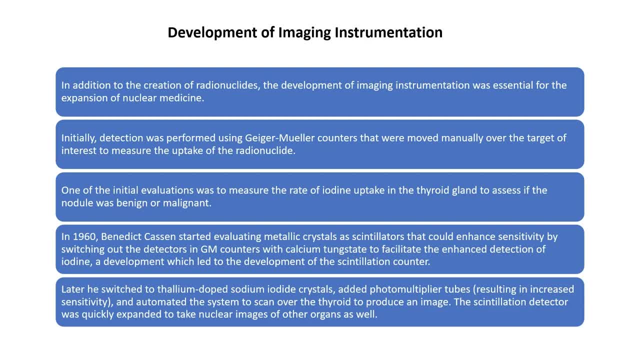 nodule was benign or malignant and in 1960 Benedict Chazen started evaluating metallic crystals as scintillators that could enhance sensitivity by switching out the detectors in GM counters to calcium tank state to facilitate the enhanced detection of iodine and development, which lead to development of 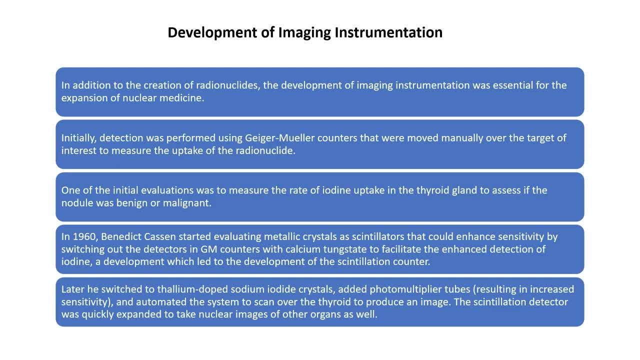 scintillator counter later switched to thallium doped sodium iodide crystals, added PMTs and automated a system to scan over the hydrate to produce an image, and that's the scintillation detector. was quickly expanded to take nuclear medicine images of other organs. 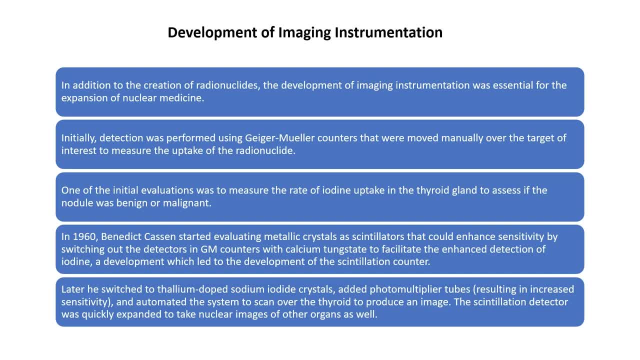 as well. so that's how the development of imaging instrument took place, from GM counter to scintillation detector, from calcium tank state to sodium iodide crystals added to PMTs, and also automation of the same to take image of other organs as well. so that's how things changed with time. so 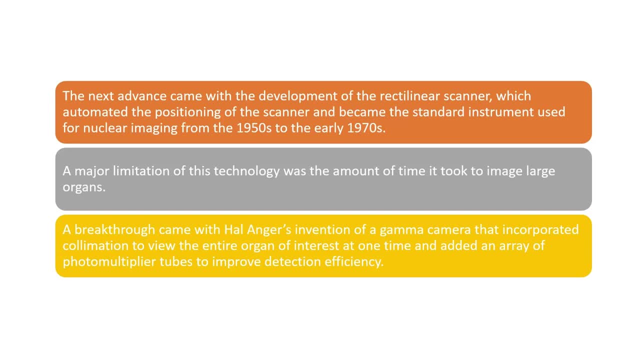 the next advancement come with the development of red kilomer scanner, which automated the scintillation detector application by their partner, GM counter. and the next advancement come with the development of Rad-Kili net scanner, which automated the the positioning of the scanner and became the standard instrument used for. 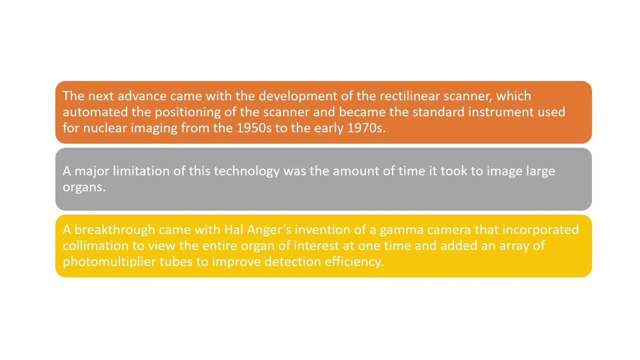 nuclear imaging from 1950s to 1970s. but the main limitation which this technology had is about the time it consumed. and a breakthrough came when Hall Enger invention of gamma camera that incorporated collimation to view the entire organ of interest at one time and added an array of photomultiplier. 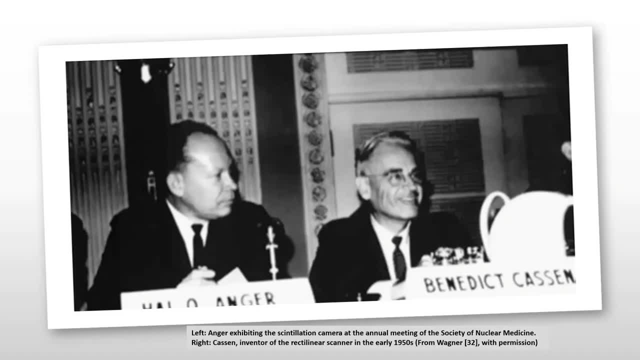 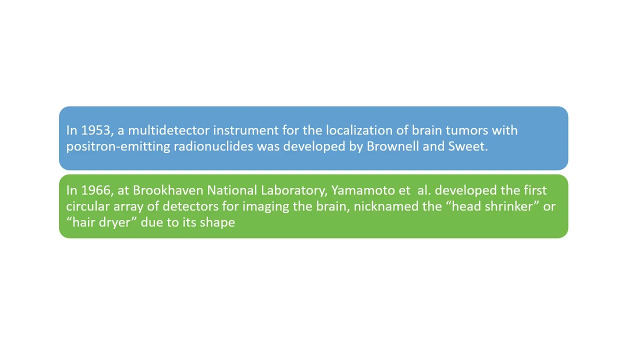 tubes to improve detection efficiency, and that's Hall Enger and Benedict Chazen, in the annual meeting of the Society of Nuclear Medicine. and in 1953 a multi-detector instrument for the localization of brain tumors with PET radionuclides were developed by 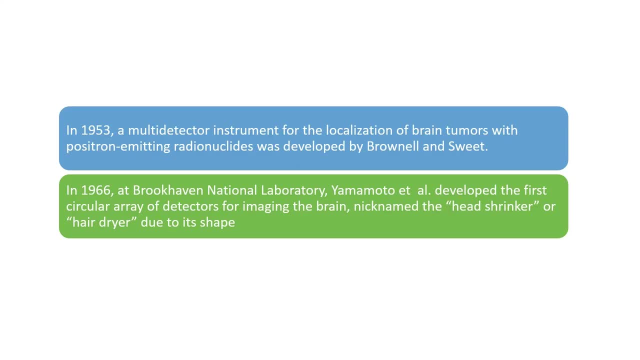 Brunel and Sweet, and in 1986 at Brookhaven National Lab, they developed the first circular array of detectors for imaging the brain, named as HEPA. HEPA is a multi-detector instrument for the localization of brain tumors. HEPA is the first multi-detector instrument for localization of brain tumors, as we can see over here. 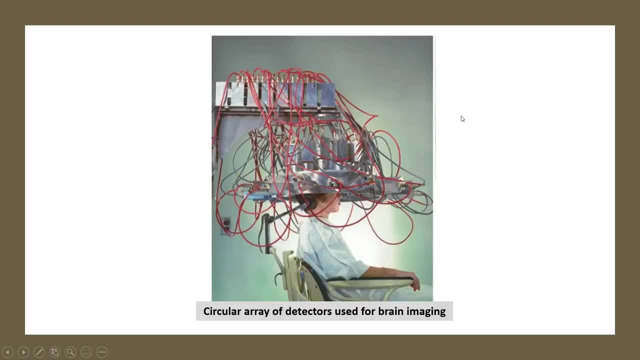 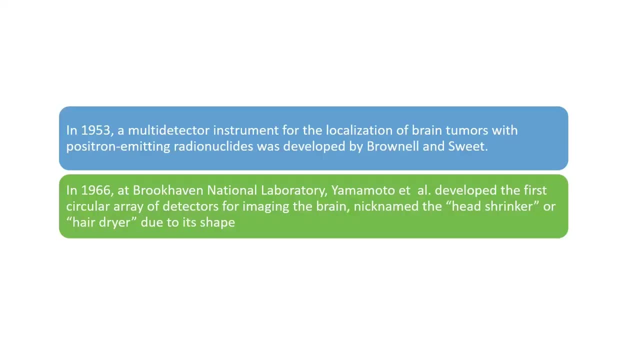 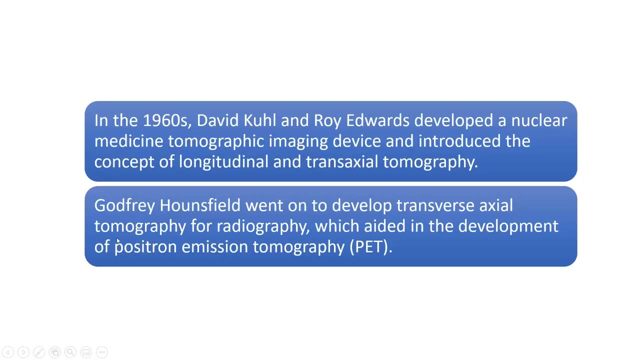 that's the possibility of a brain tumor over here and that's the circular array of detectors used for brain imaging, also being called as HEPA because of its shape. So in 1960s, David Cull and Roy Edwards developed a nuclear medicine tomographic imaging device and introduced the concept of 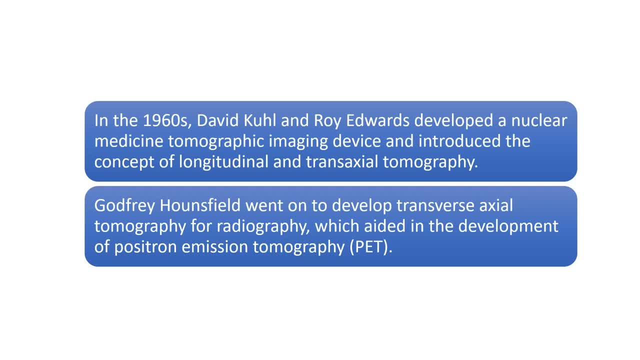 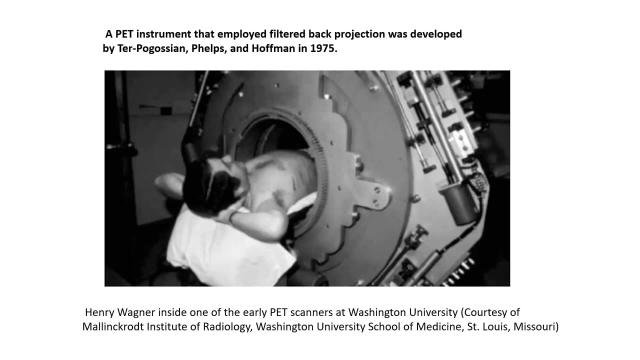 longitudinal and transaxial tomography and this was announced by by Hornsfield when he developed the transverse axial tomography for radiography, which aided the development of PET, and that's the first PET instrument that employed the filter back protection. and that's how it looks like and that's Henry. 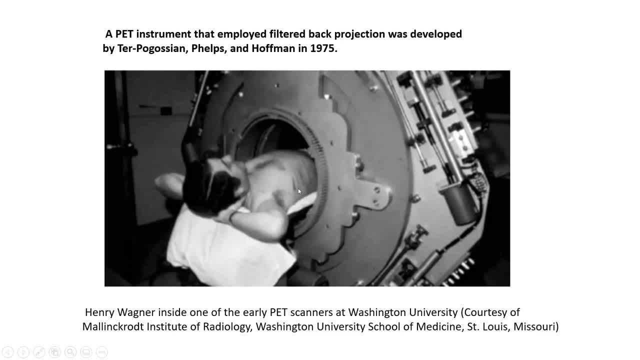 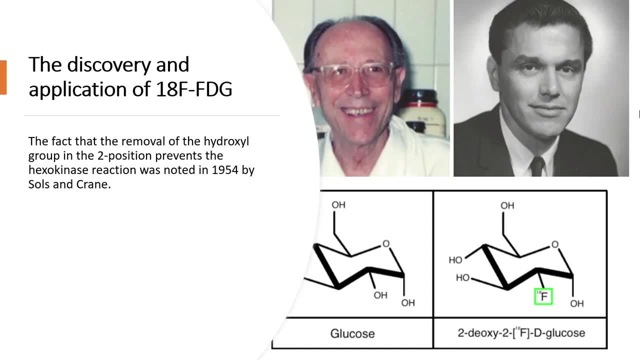 Wagner inside the early PET scanners at Washington University. so now let us talk on the discovery and application of F18 and FDG. so if you look at the structure of glucose and and FDG, both of the structure looks very, very similar, but the main difference lies at the second carbon position in which you can 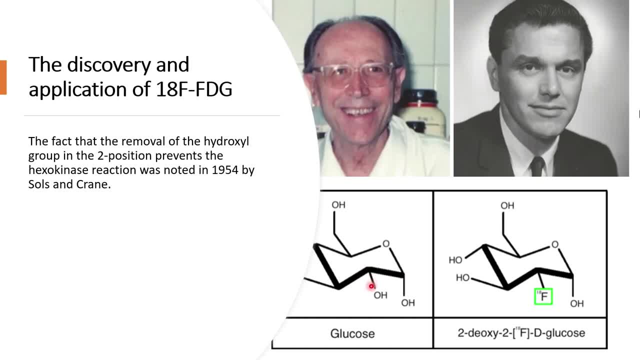 see, in glucose there is an hydroxyl group, but in in in FDG there is an F18 and this F18 is in positron ammeter and decays by positron emission and these FDG is being used to study glucose metabolism in human in in in 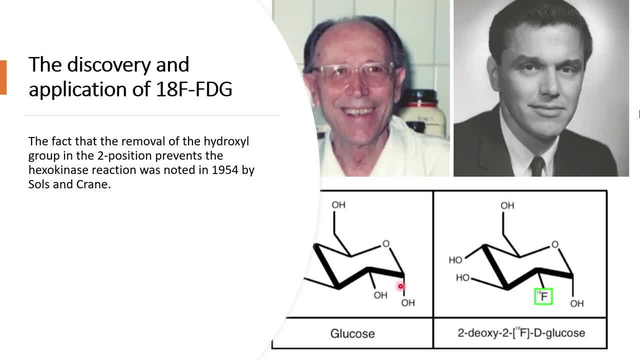 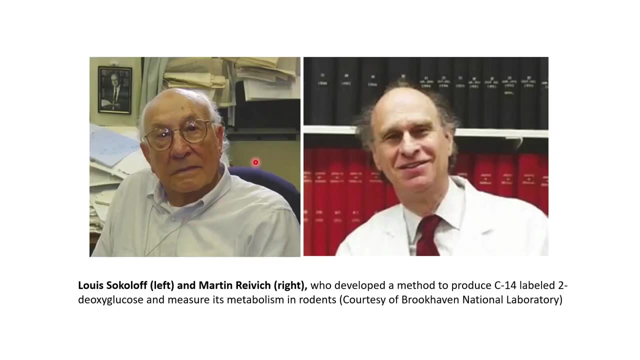 human beings. so the fact that removal of these hydroxyl group on second carbon position prevents the hexokinase reaction was noted in 1944 by this two group of people, Salz and Crane. and based on this idea, these two group, these two people, Louis and Martin, developed a method to produce C14 labeled to 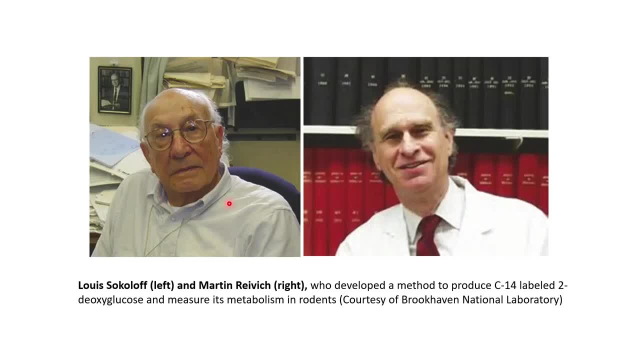 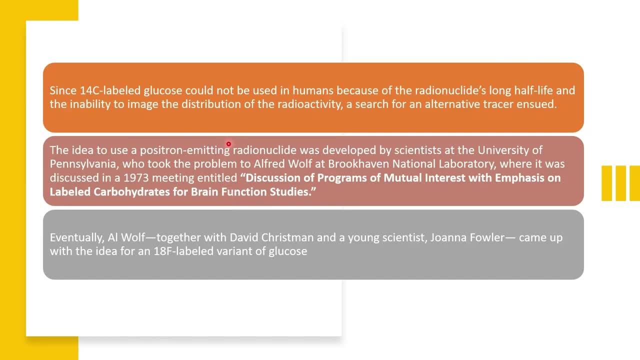 deoxyglucose and measure its metabolism in rodents. but C14, as you know, it's a very large half time of 5700 years, so it cannot be used in human because of its long half-life and its inability to image the distribution of the radioactivity as such. for an alternative, 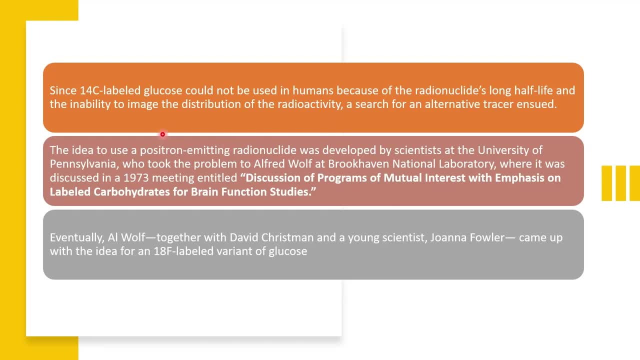 of tracer started ensuring. and finally, the idea to use a positron emitting radionuclide was developed by scientists at University of Pennsylvania, who took the problem to Alfred Ulf at Brookhaven National Lab, where it was discussed in 1973 and in a meeting entitled discussion of programs of mutual. 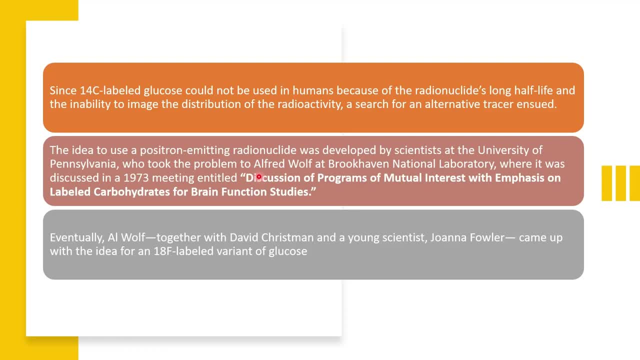 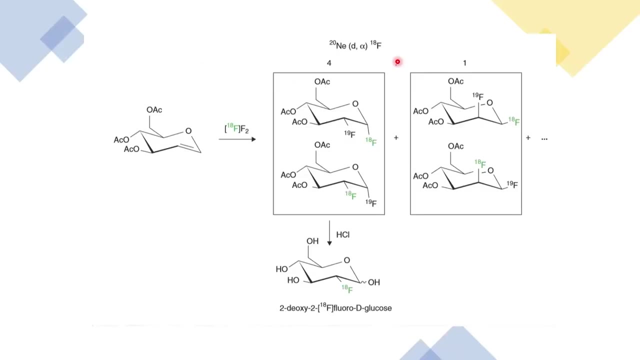 interest, with emphasis on level carbohydrates for brain function imaging, brain function studies and eventually he came out with a great idea and to produce 18 F labeled variant of glucose. and that's the process by which he produced F18, FDG- that's bombarding neon with deuterons and 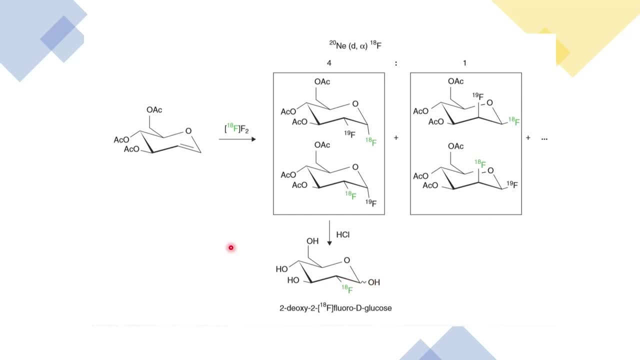 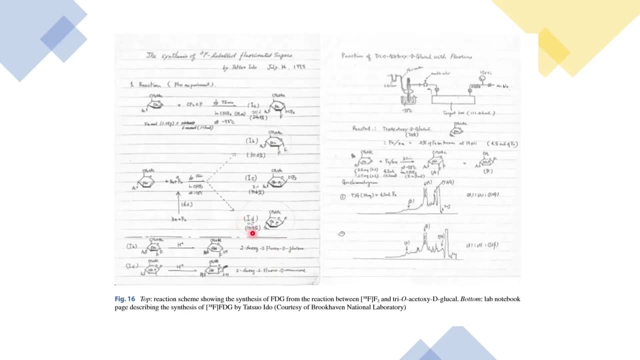 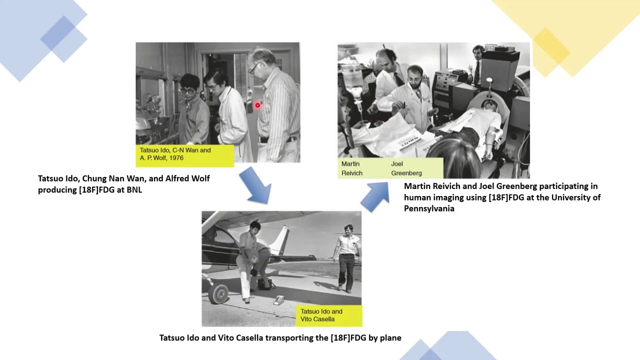 getting F18 and this F18 was processed further to get to the state and these were being: and that's the lab copy, lab lab notebook describing the synthesis of FDG and and that's how this FDG was in, produced in Brookhaven National Lab by this group, by this group of people. so, but now they have prepared. 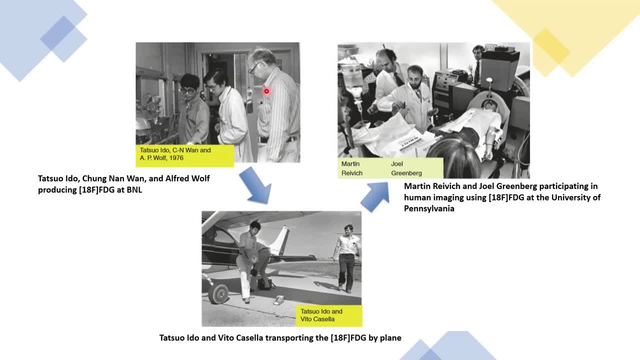 this FDG but it has to be tested, it has to be, it has to be mazed also. so at the time the closest PET center was in Philadelphia, so FDG need to be transported from the Brookhaven lab to the Philadelphia so that it can be mazed in. human logistics work were pretty interesting. FDG was. 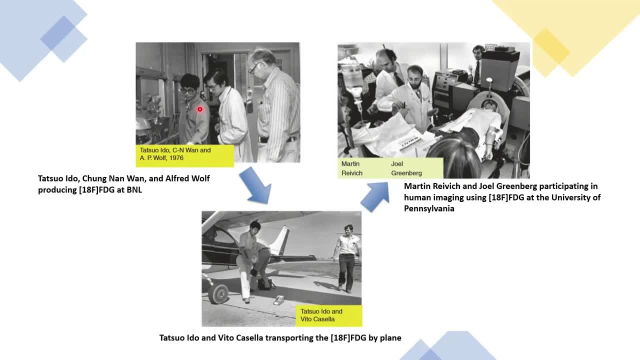 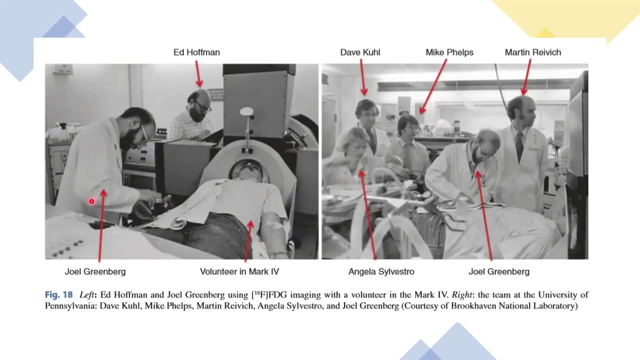 made in Brookhaven, backed by health physics group, are driven to the local nearby airport, put on a small four-person plane and flew from Philadelphia Airport and flew from Philadelphia Airport and driven to the University of Pennsylvania and where it can be injected. so that's how, is how and that's how it goes on. so, and that's the group of people, that's. 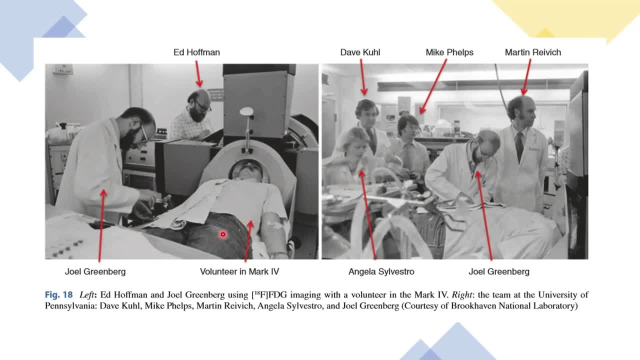 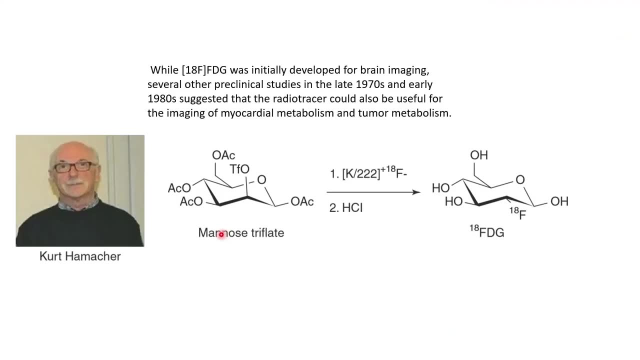 the volunteer- and that's how it all started- for production of FDG in Brookhaven National Lab and imaging studies at University of Pennsylvania. so while the initial development of FDG was initially developed for for brain imaging, but several other preclinical studies in the late 1970s and early 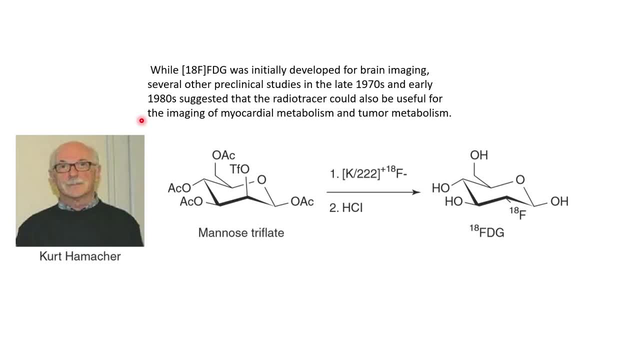 1980s, suggested that this tracer can be used for imaging the myocardial metabolism and tumor metabolism also. and then, by means of this person, mr dr Kurt, he produced a new process of, of producing FDG through a nucleophilic process through mannose. 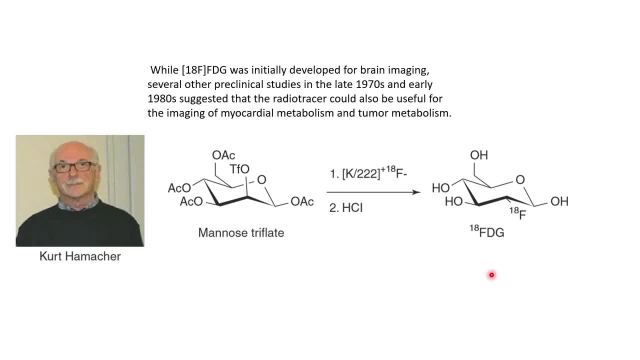 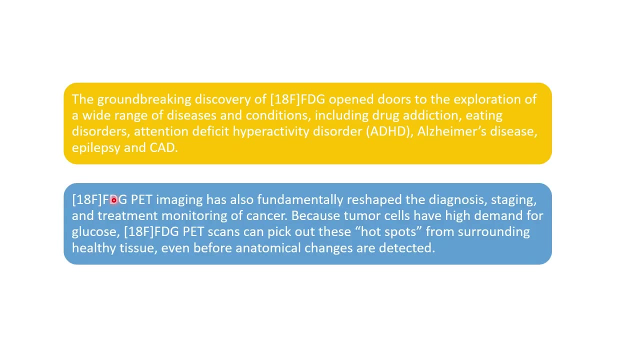 differently through this process to get to FDG. we'll talk about even you talk about the production of FDG, so we'll talk about this reaction also. but this guy produced a greatest process of producing FDG with highest yield niche in a short duration of 50 minutes. so and this groundbreaking discovery of 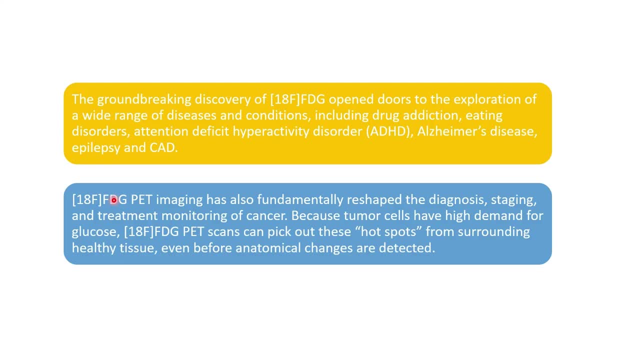 FDG opened doors to the exploration of a wide range of disease and conditions, including drug addiction, eating disorders, attention, attention deficit hyperactivity disorder as a my disease, epilepsy and CAD. and these FDG pet imaging was also very important for imaging, for for the diagnosis, staging and treatment monitoring of cancer, because cancer 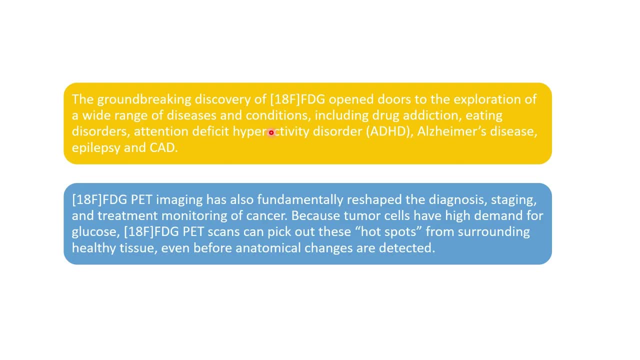 are metabolically more active and they take more FDG than the normal cells and they are being that can be seen as hotspot from surrounding healthy tissue, and that's the advantage of FDG. also, it has great implications in a wide range of disease, from these group of disease to even cancer diagnosis, staging and 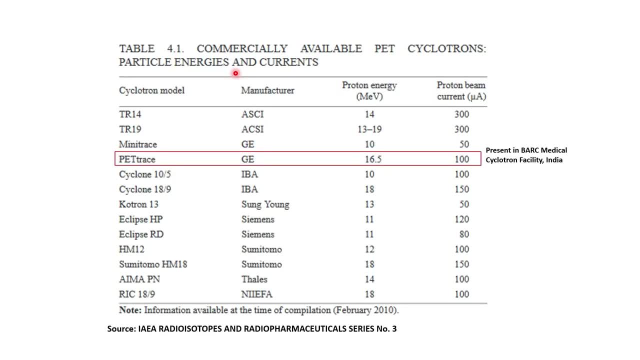 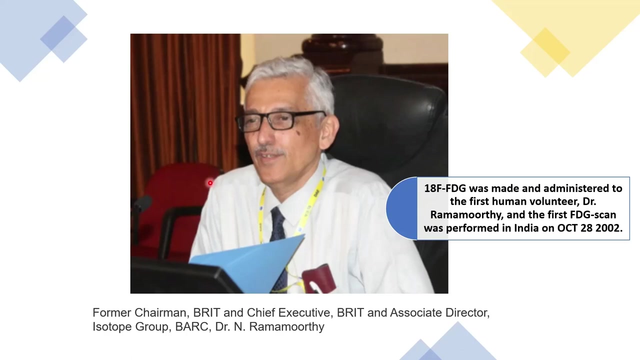 treatment, monitoring of cancer. and these are the group of cyclotrons available across the globe for production of FDG, and that's the batteries manufactured by GE is present eat in BRC medical cyclotron facility in India which has an photon energy of 16.5. and that's Dr Ramamurthy, who was the former.